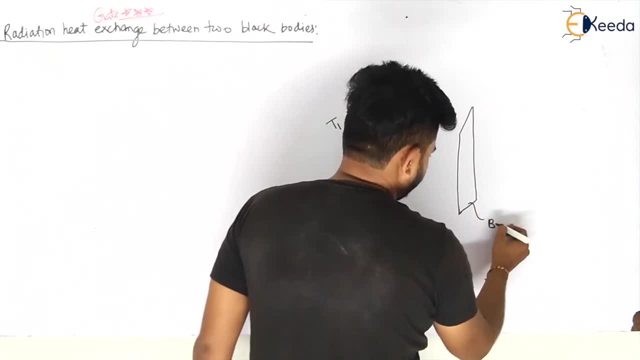 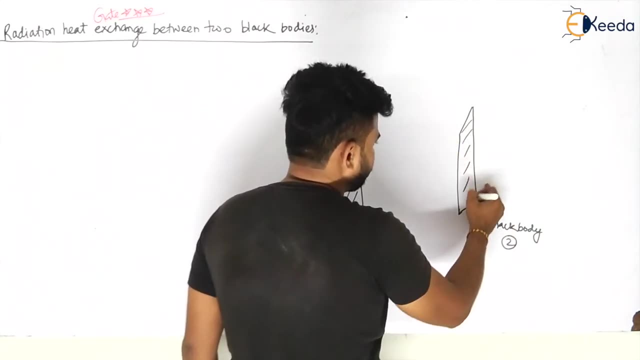 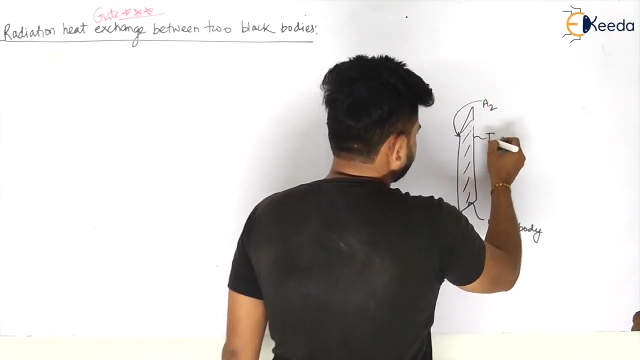 That is black body. 2. Like black body. Okay, this is having some area from this side to be like A2.. And temperature? let us take the surface. temperature is T2.. Okay, now let us understand carefully what is happening. 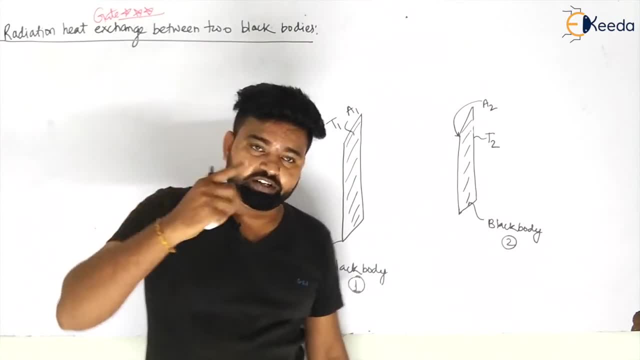 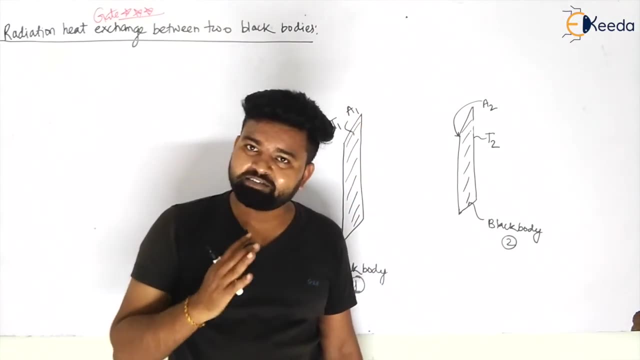 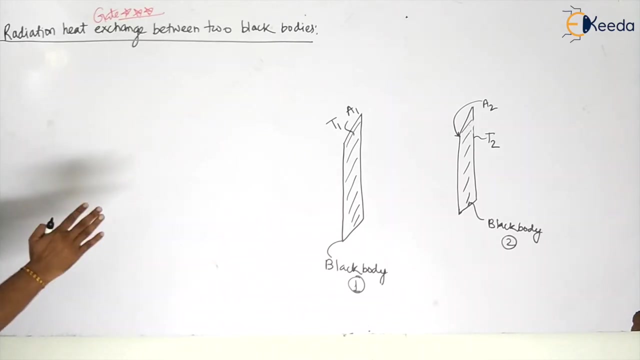 So body 1, if I will analyze only body 1, let us focus on this body, only this body only. So this body will emit some radiation. So can I have a total emissive power of body 1?? Yes, I can have the total emissive power of the black body 1,. my dear students, 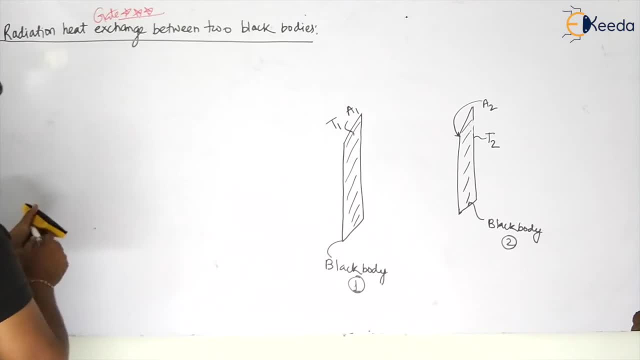 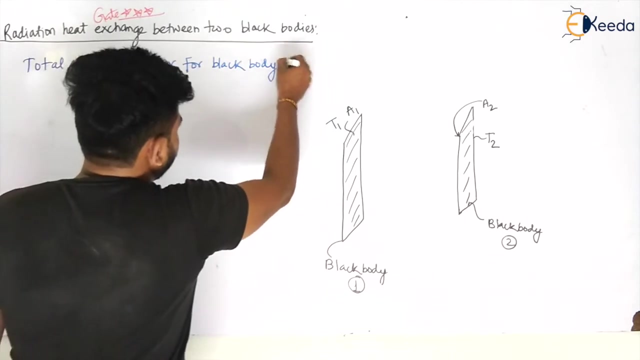 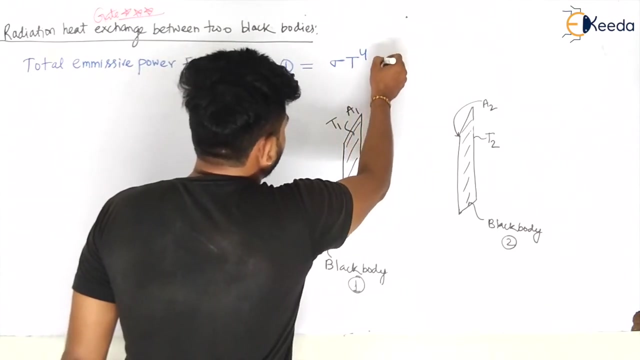 So total emissive power or total radiation? total emissive power, power for black body 1, body 1 is given by what, my dear students, Is given by sigma T to the power, 4 watt per meter square. Calvin to the power 4,, my dear students, Yes or no Calvin to the power 4?. 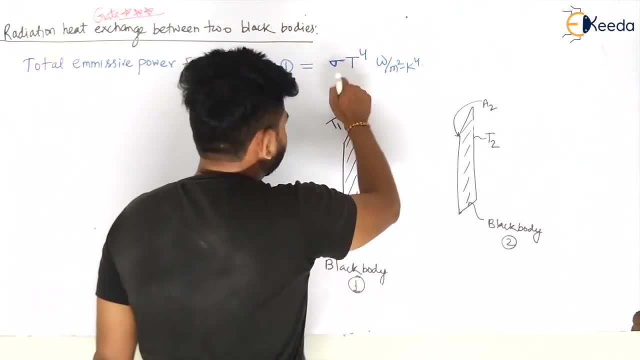 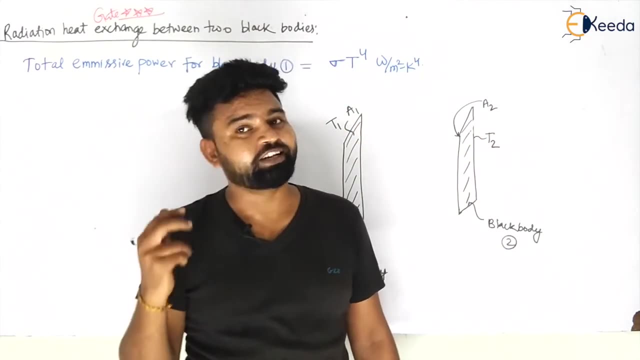 Now, this is for the per unit area And this is coming from where This is coming from your. when you are summing this over, all over the wavelength, then you are getting this. okay, Now, what will be the total emissive power? This will be per unit area. we are taking. 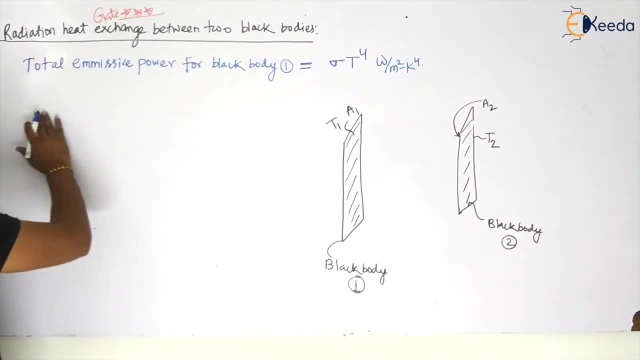 Now let us see. let us see. So what will be the total emissive power That is for per unit area? you said you should take per unit area, So total emissive power. total emissive power for body 1,. 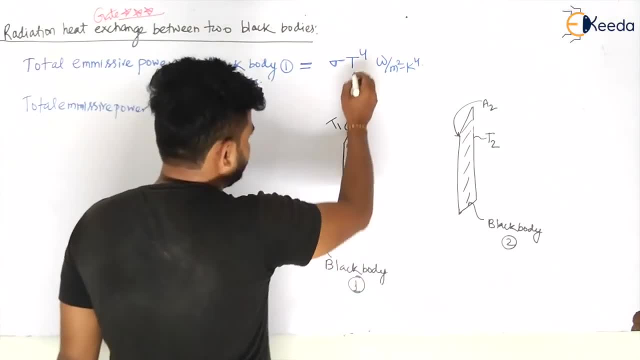 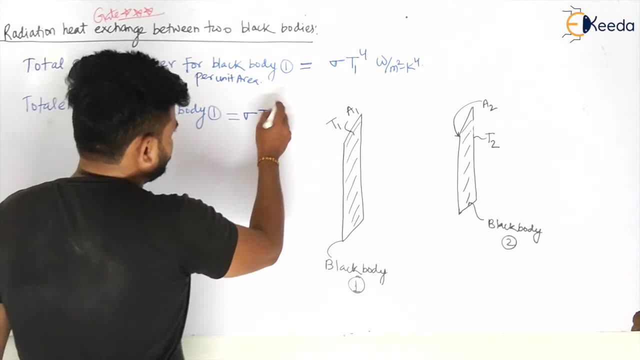 it will be equal to, as you are talking about the body- 1, so let us take T1 to the power 4.. So if I will take the total power, this will be sigma T to the power 4, multiplied by K1,, multiplied by K1,, my dear students, 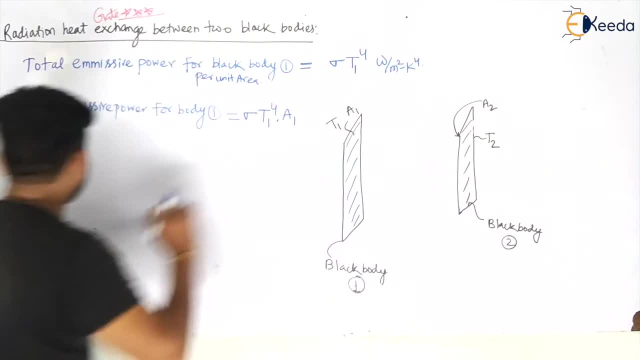 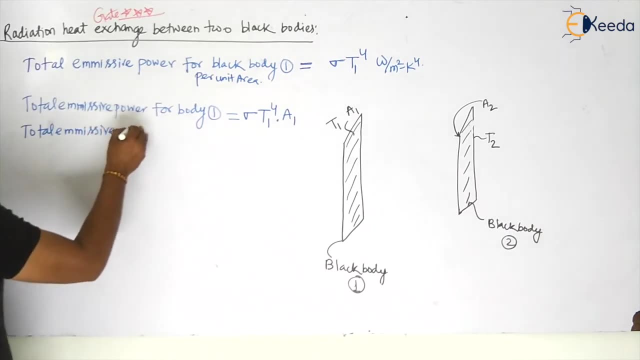 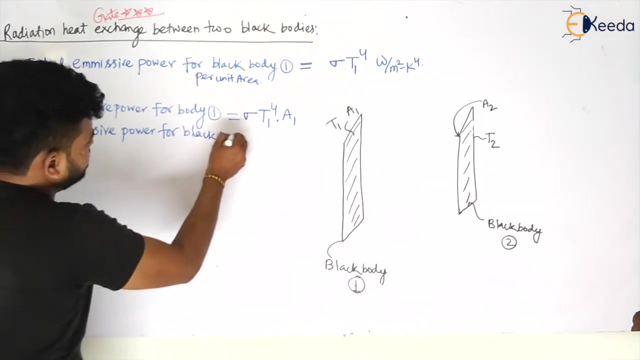 So can I directly take for body 2?? Yes, So the total emissive power, total emissive power power for black body 2.. Black body 2 or surface 2 will be given by sigma T to the power 4 and this will be watt per. 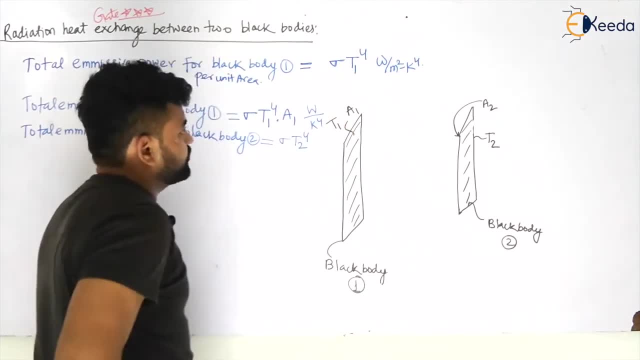 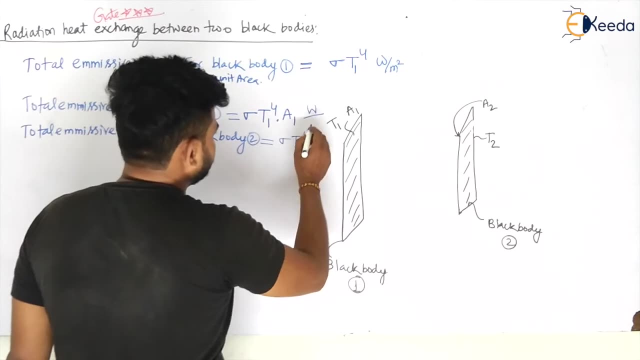 Kelvin to the power 4 and this will be watt. We can, we should directly take watt per meter square. okay, Watt per meter square, this will be in watt, okay, And this will be A2,, my dear students, this will be A2.. 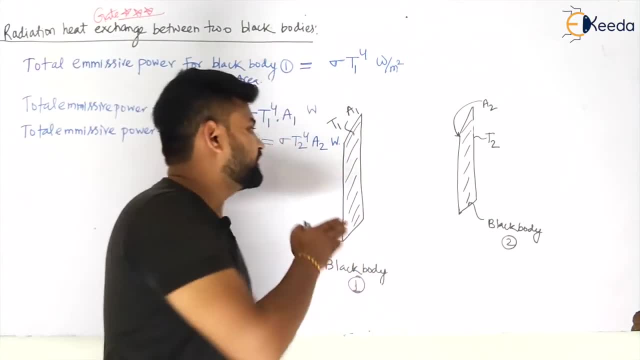 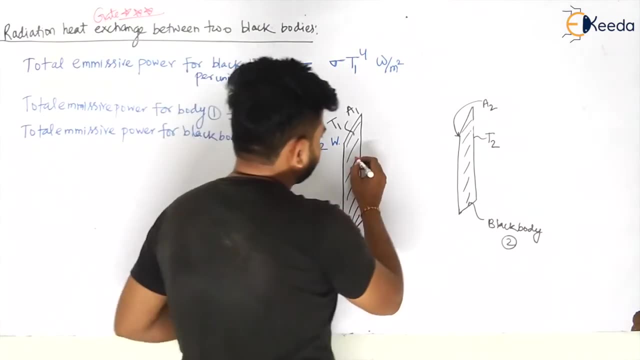 So now this may be happening, that this is radiating, radiation in all directions, okay, And some fraction may be reaching on 2.. Let us take it So. this is again, we are going to the shape factor, my dear students. 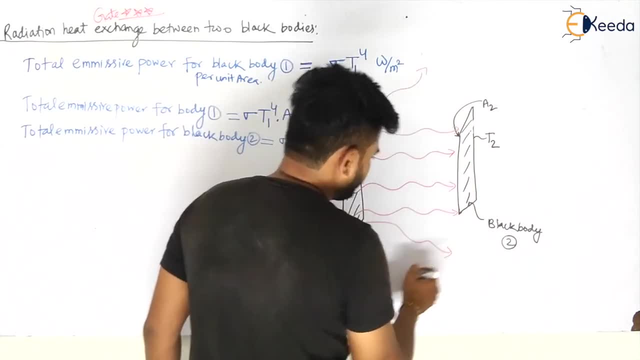 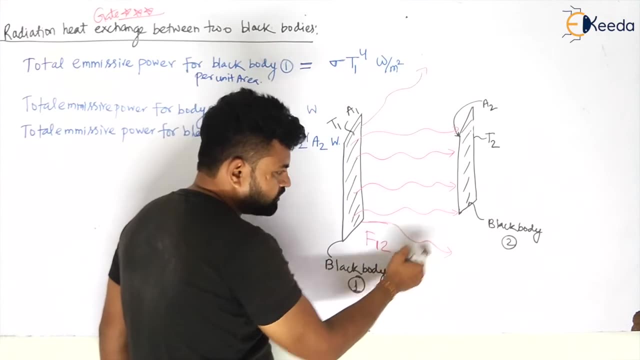 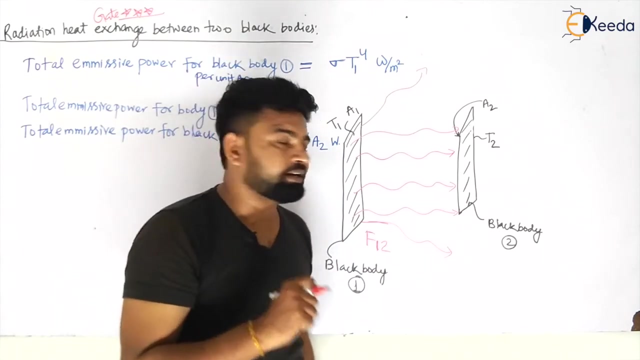 And some is going out, my dear students. So what will be the shape factor for this? That is, living surface 1.. And falling on surface 2,, my dear students, Falling on surface 2.. So can I calculate the radiation absorbed by the body 2?? 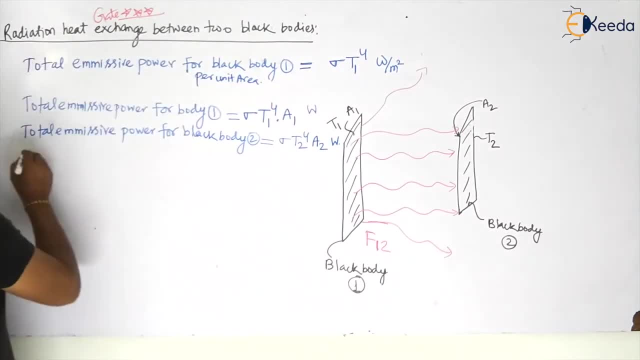 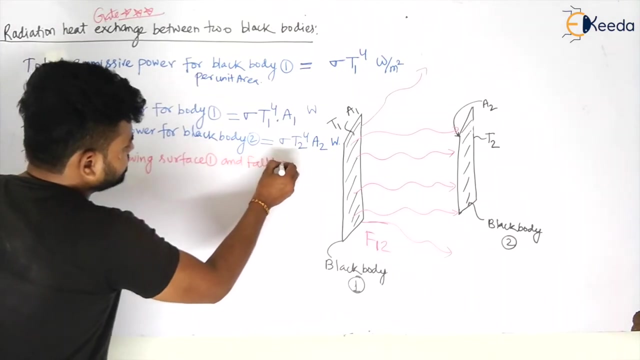 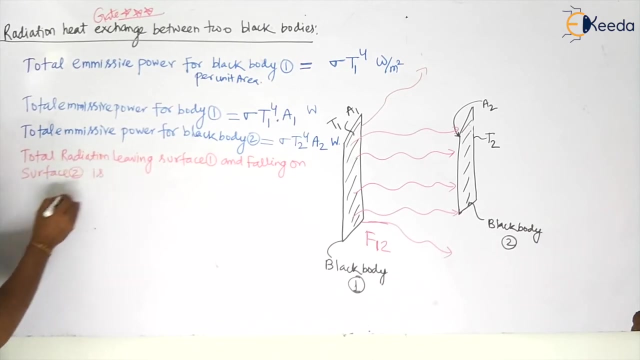 Yes, I can calculate. Yes, let us see So. total radiation living 1.. Total radiation living surface: 1. And falling on 2. On surface 2. Is nothing, but what? Let us take it, This will be given by some self-impactor. you have to multiply. 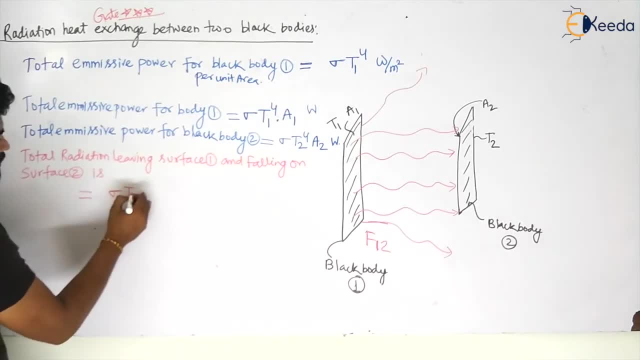 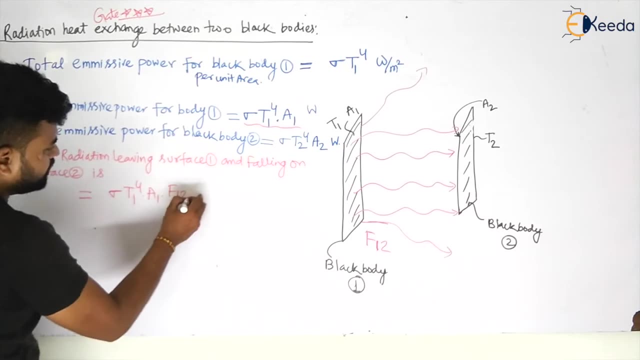 So this will be given by equal to sigma T1, to the power 4, living 1.. So total radiation living 1 is this X into A1 multiplied by F1 to my dear students. So that is the total radiation which is living 1 and falling on the 2.. 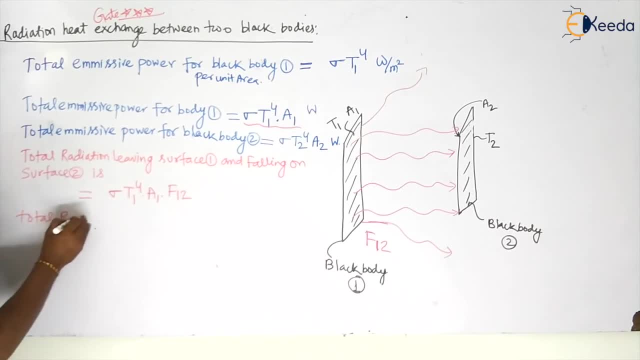 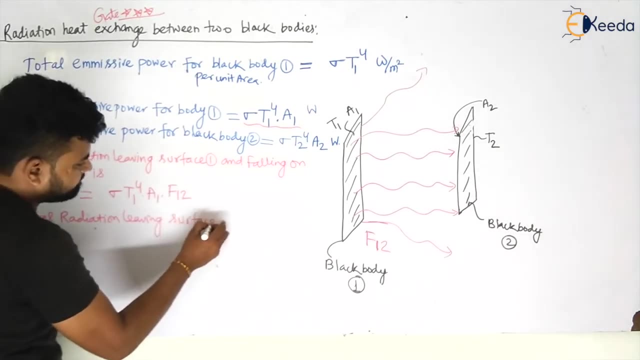 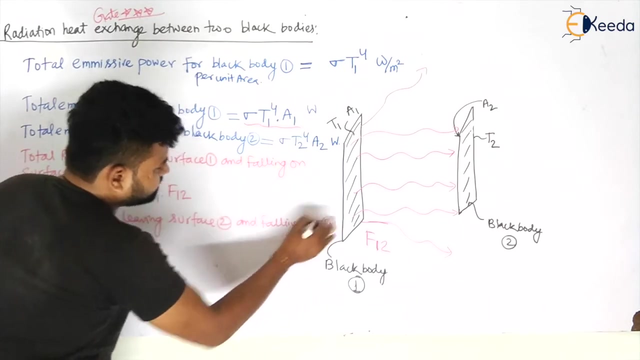 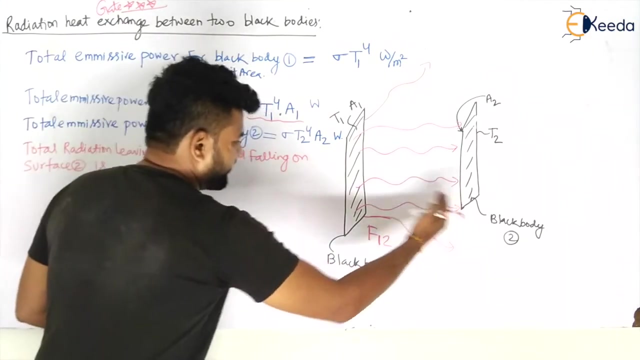 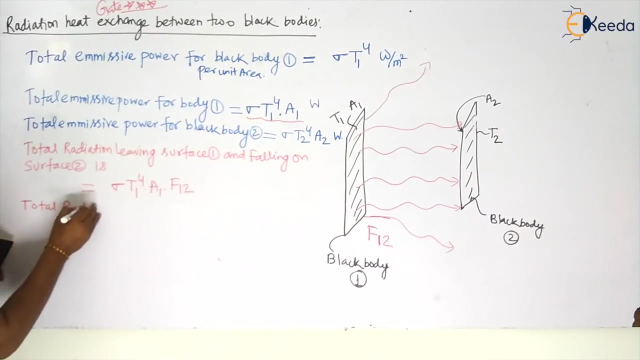 Similarly can we calculate total radiation: Total radiation living 2, living surface 2 and falling on surface 1.. So this will be So the total radiation, which is living surface 2 and falling on 1 will be total radiation. 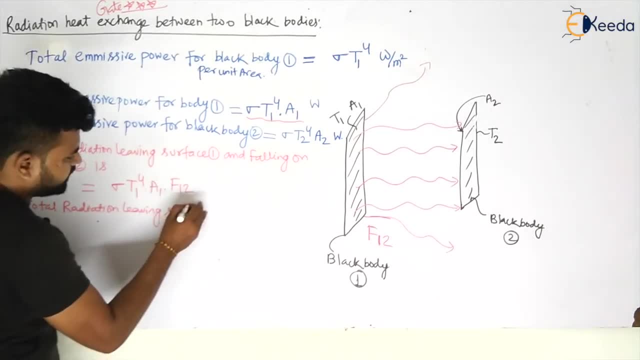 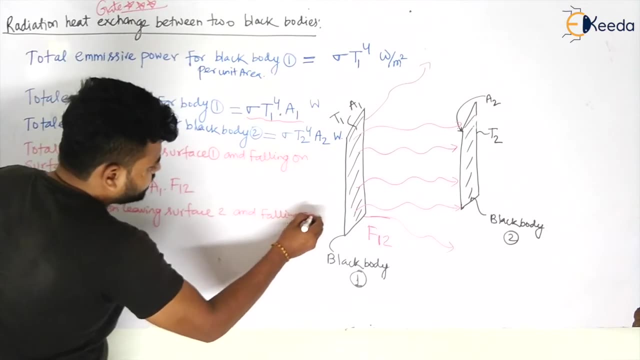 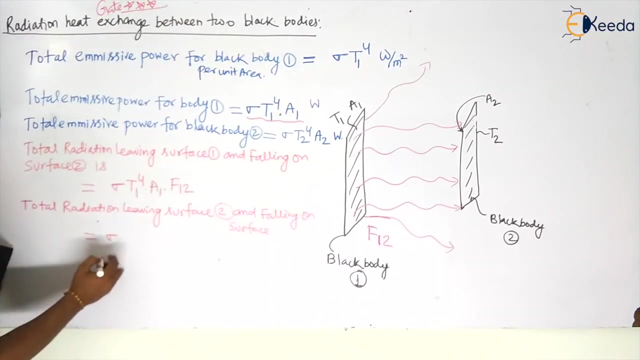 Living surface 1 or living surface 2,, my dear students. Surface 2 and falling on surface 1.. Surface 1,, my dear students, Will be what? This will be nothing but sigma. That is living 2,, my dear students. 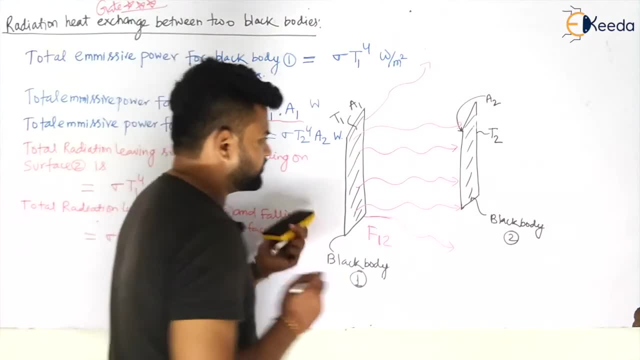 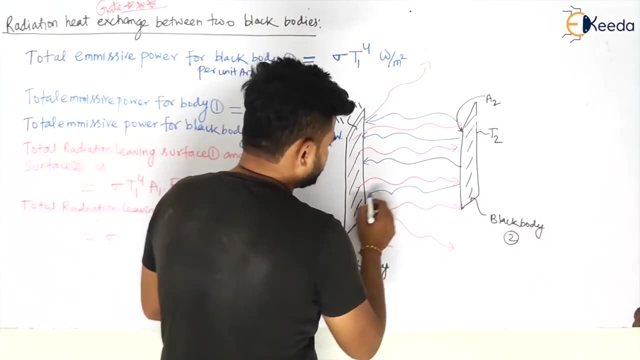 That is living 2.. 2 means that which is coming out from this and falling on 2.. So what will be the view factor for this or shape factor for this? So that is living surface 2 and falling on 1,. my dear students, 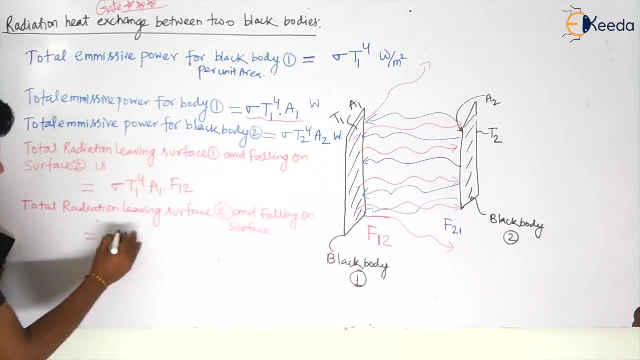 So this will be given by sigma T to the power 4.. Okay, Multiplied by A2 into F21,, my dear students, F21.. So this is which is living 2 and falling 1.. This is which is living 1 and falling 2.. 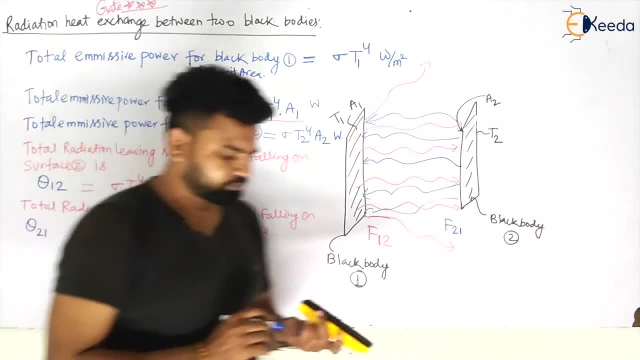 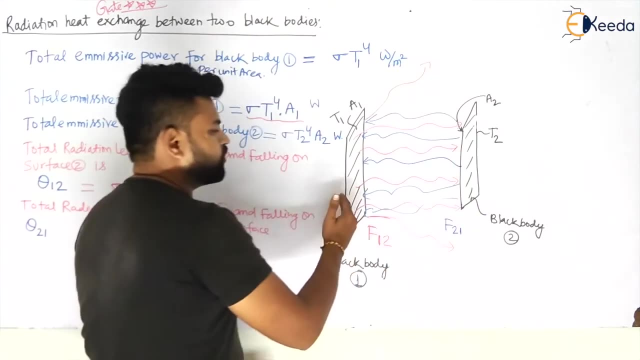 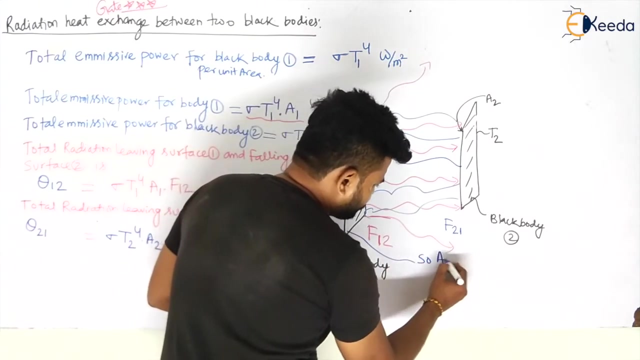 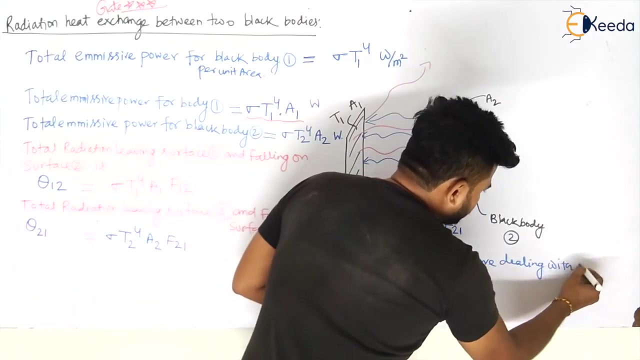 So that is an area. So this is Okay Now as we are dealing with the black bodies. So whatever the radiation will be coming from 2 and falling on 1 will be absorbed by this body surface, 1.. So As we are dealing with dealing with black bodies, black bodies, 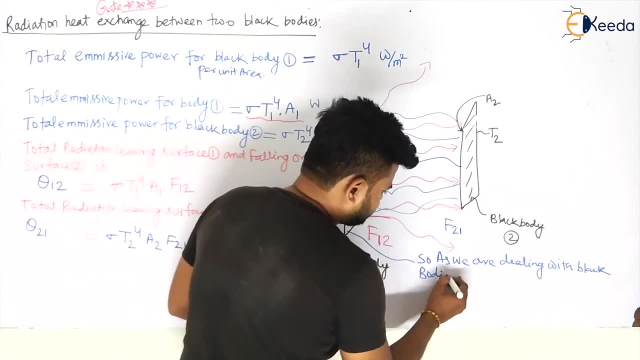 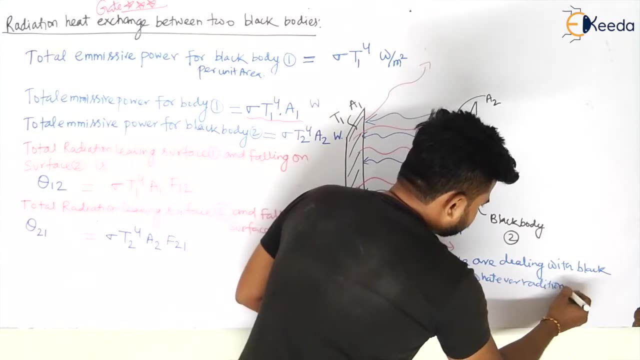 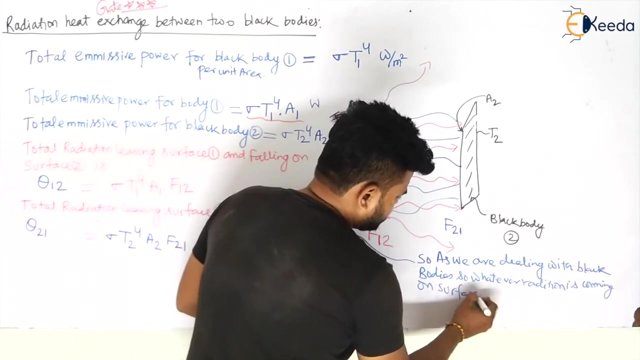 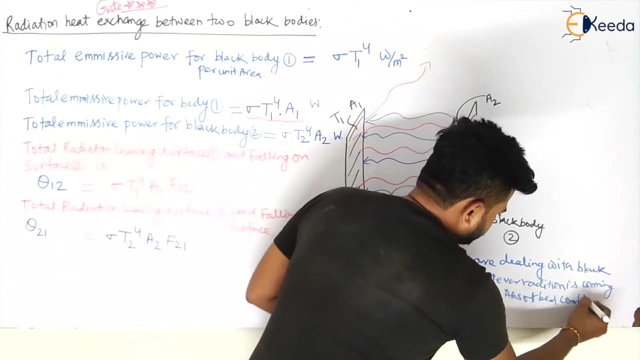 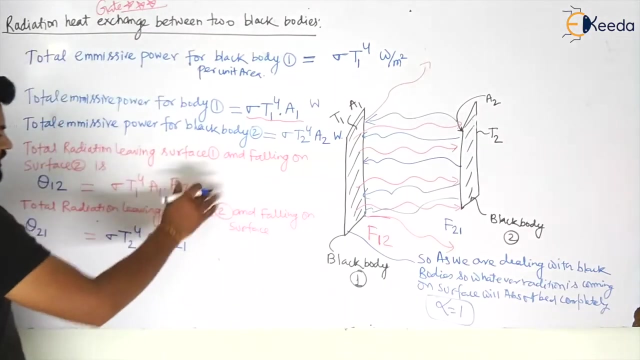 So, whatever radiation is coming, coming on surface, on surface, will be absorbed completely, will be absorbed completely. will be absorbed completely, my dear students. completely how? because for black body, your alpha is equal to one. so whatever the radiation will come, it will absorb completely. let us take that is alpha two. let us take that is alpha one. and 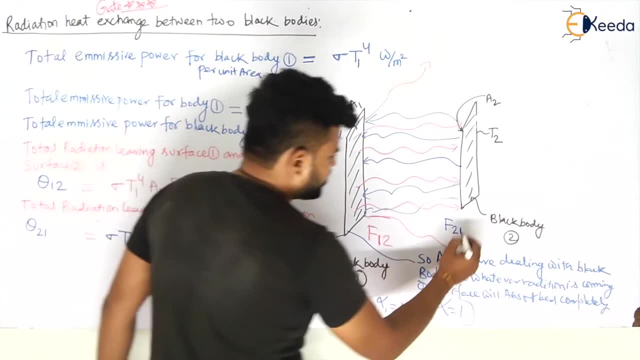 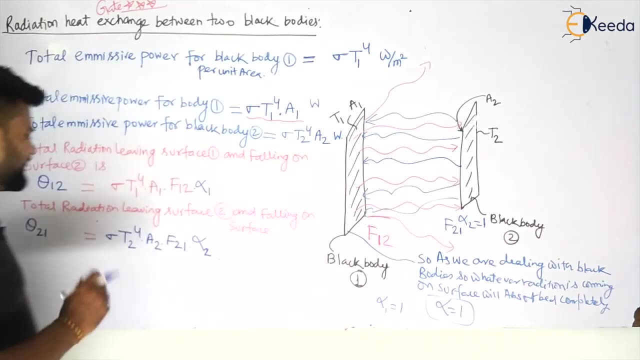 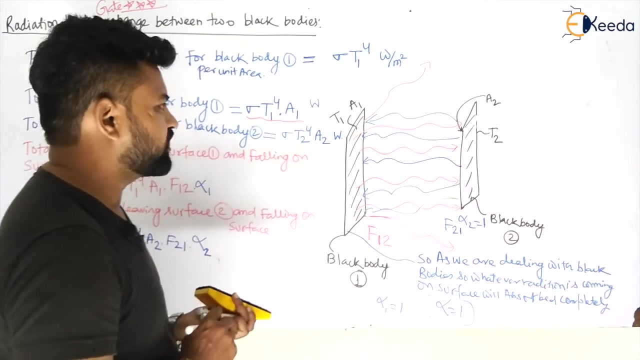 in our case, alpha one and alpha two is equal to z or equal to one. my desperate, because we are dealing with the black bodies now. can i calculate the net radiation heat exchange between two black bodies? yes, now the net radiation heat exchange between these two surfaces, these two surfaces. 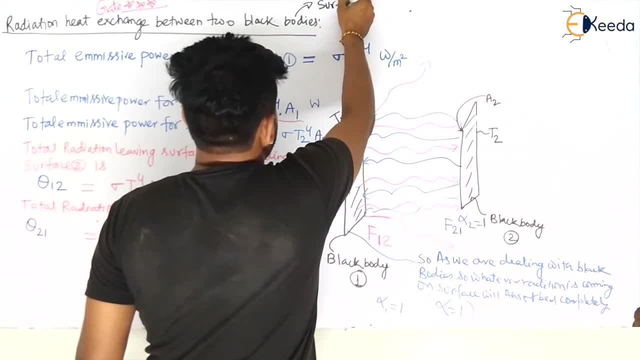 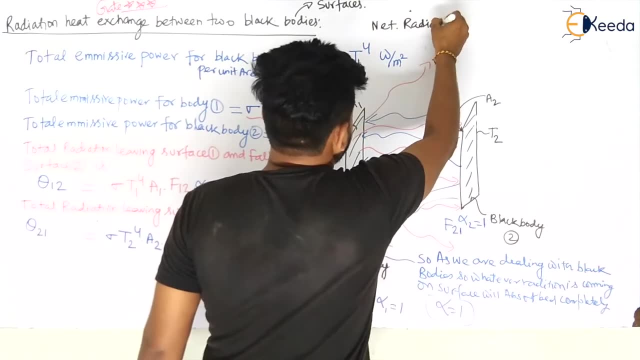 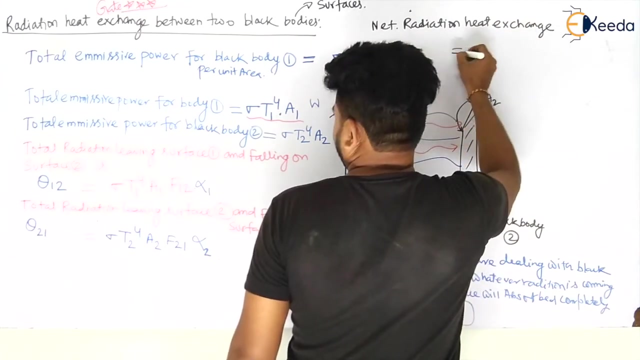 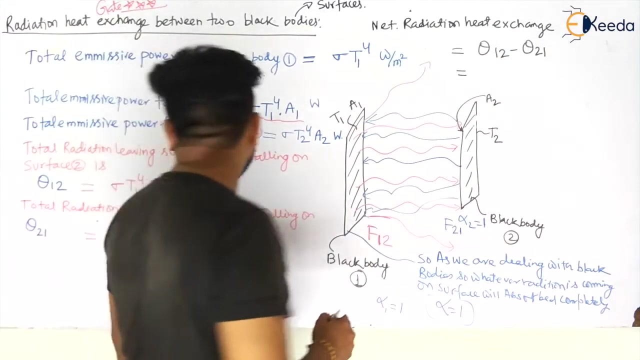 you can also talk about the lighted surfaces. so net radiation heat action will be given by net radiation heat exchange. you will be what will be? q12 minus q21, yes or no, my dear students? q12 minus q21, so can i take? so this will be nothing. 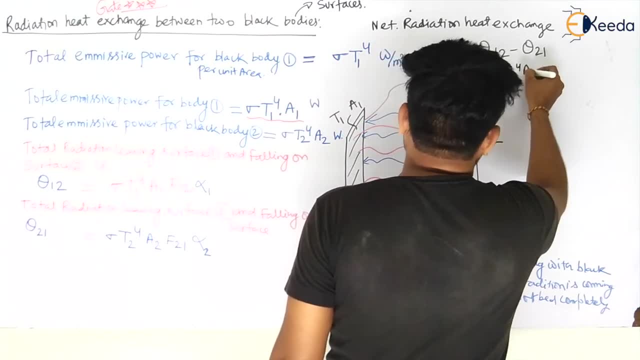 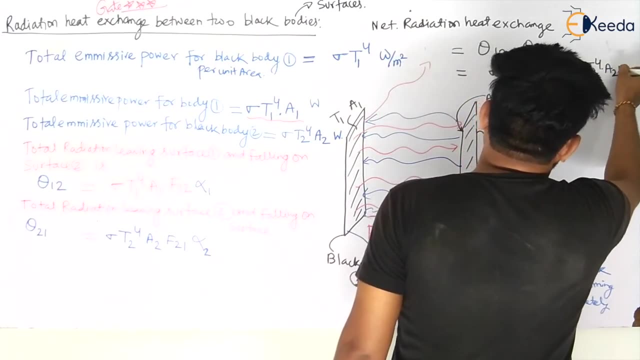 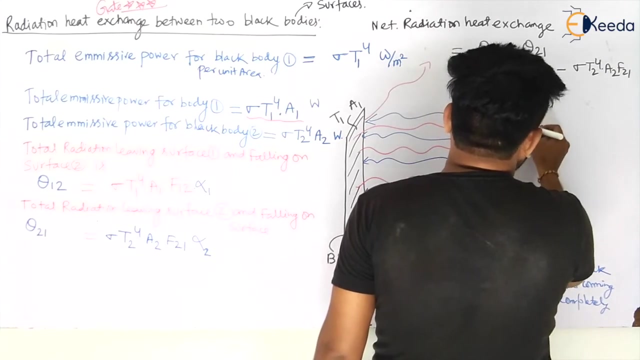 but sigma t1 to the power 4, a1, f12, minus sigma t to the power 4, that is a2, f21. and i have taken alpha 1, alpha 2, equal to 1, equal to 1. so in this case the net radiation heat exchange q net will become 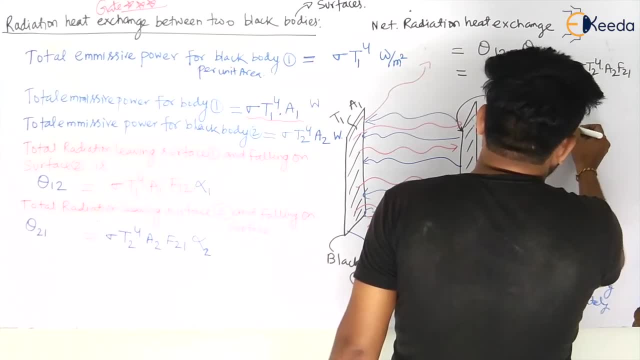 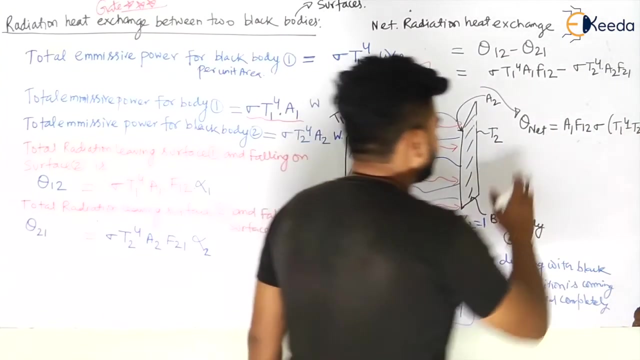 equal to that is your a1, a1, f12, into sigma, into sigma c1, to the power 4 minus t, to the power 4, my dear students, even to the power 4 minus t, to the power 4, or directly, let us right here. so let us take it. 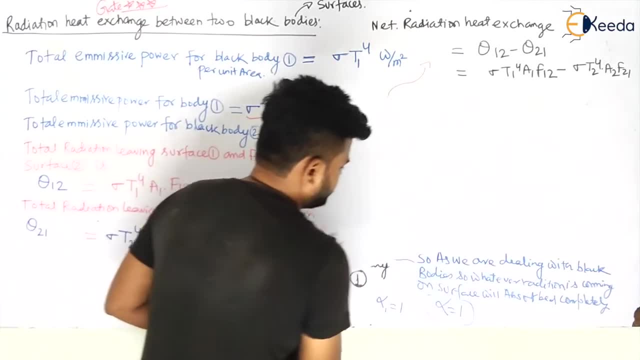 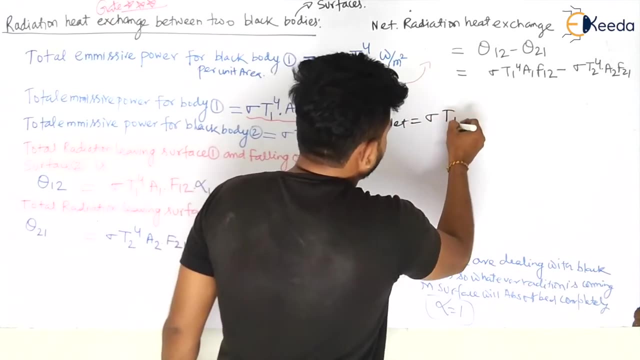 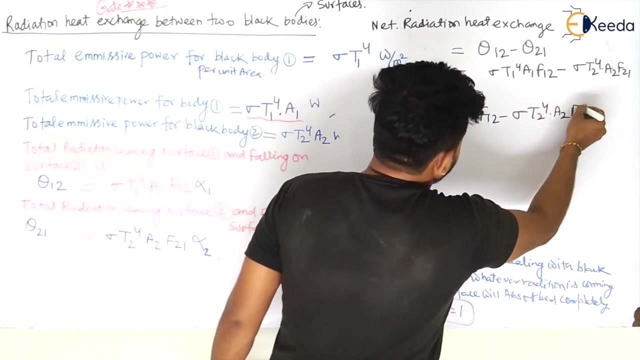 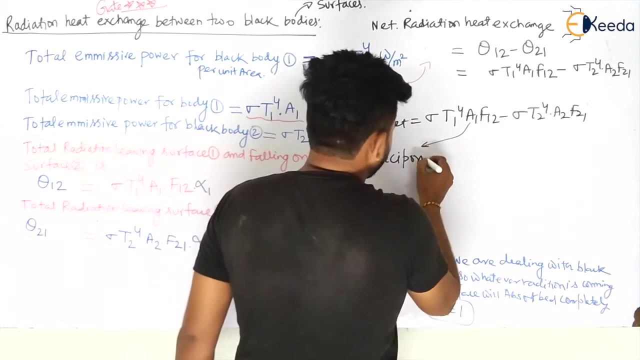 out. so the net radiation heat action will be given by, so that is q. net will be given by sigma even to the power four a, one, f, one, two, minus sigma t to the power four a, two, f, two, one. so, if i will use the reciprocity theorem, reciprocity, theorem, reciprocity. 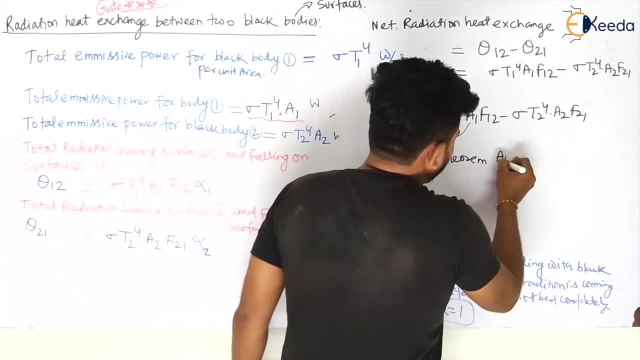 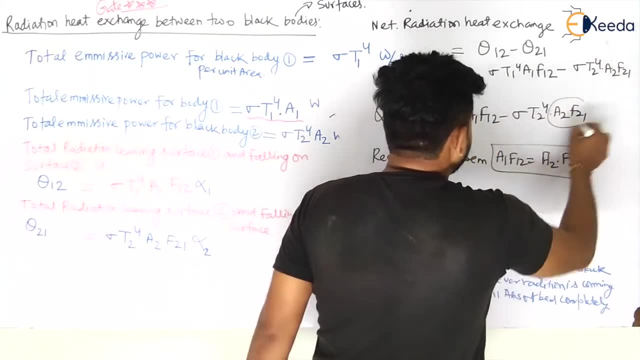 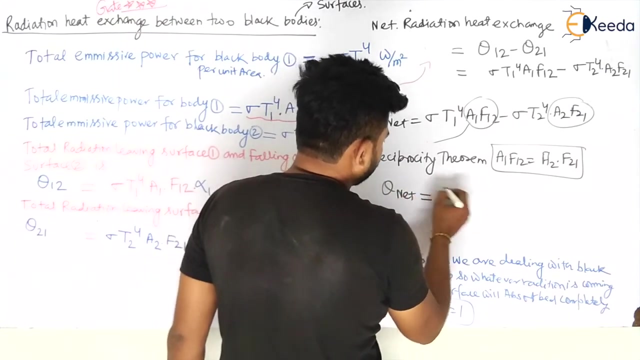 theorem what we know, that a 1, f 1, 2 is equal to a 2, 2, f 2, 1, my dear students, f 2, 1. so this part will be equal to this, yes or no? so can i write this? q net is equal to, for black bodies will be given by a sigma: a 1. 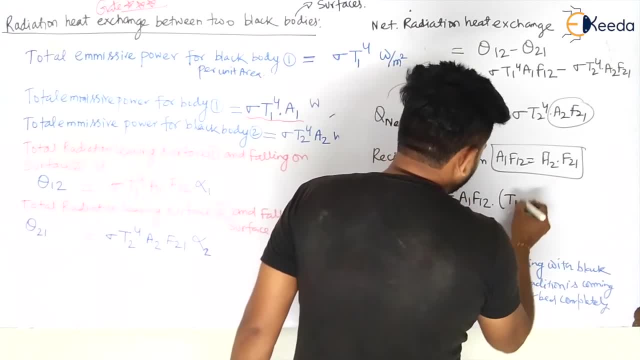 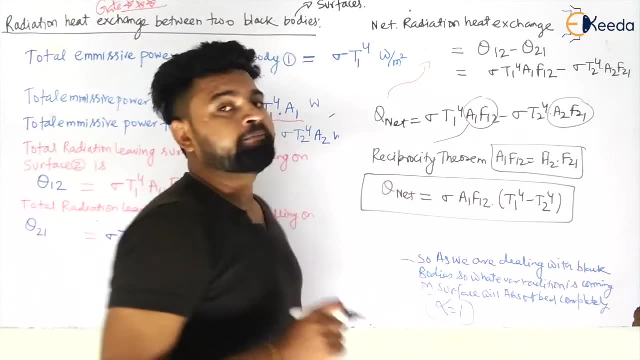 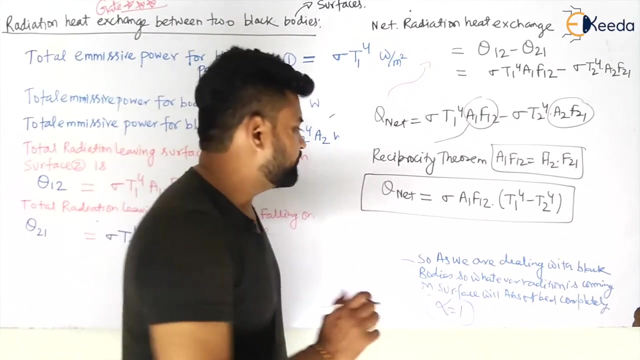 f, 1, 2, multiplied by t, 1 to the power 4, minus e to the power 4, and this will be the net radiation heat exchange between the two surfaces. my dear students, okay, so number of questions will be asked on this. if he will give you two black bodies, 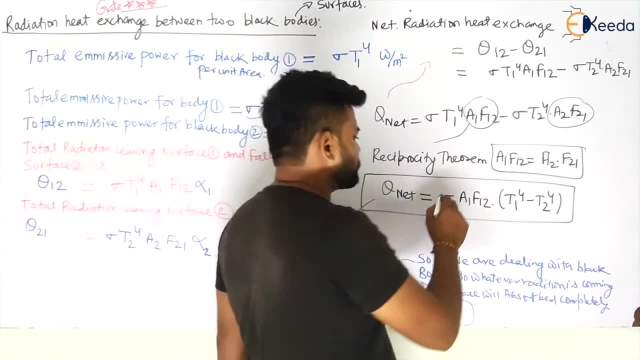 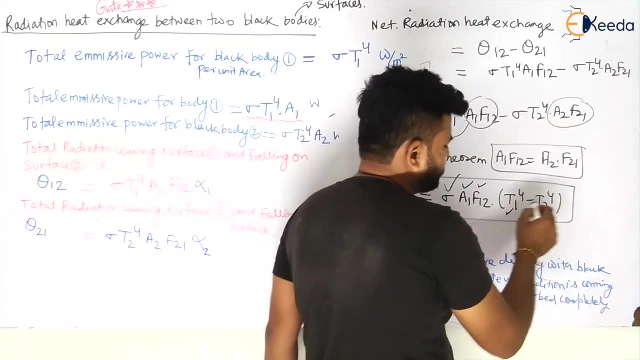 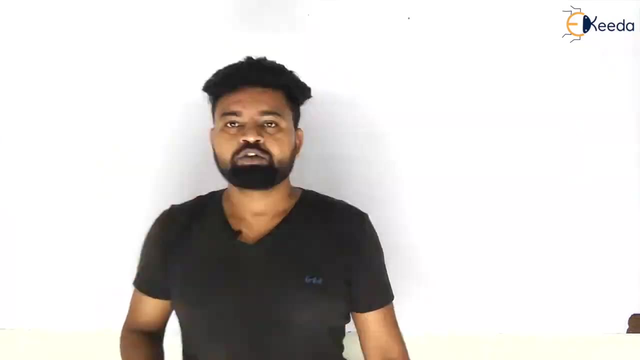 and you want to calculate the net radiation heat action, you must know the value of sigma a1, f1, 2, you will know you can calculate f12. if you know now t 1 and t 2 will be given, you can easily calculate the net radiation heat action my life created. so thank you so much, so we have. 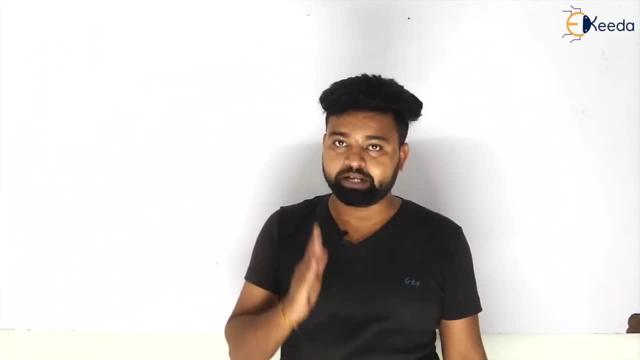 discussed about the net radiation heat exchange between the two black surfaces or two black bodies, my dear students. so now we have. you've come across the f1 and f2, so let us take a look at the previous equations. you will be asked on the web also, super-unf인을, this super uniform. so number of commissions. 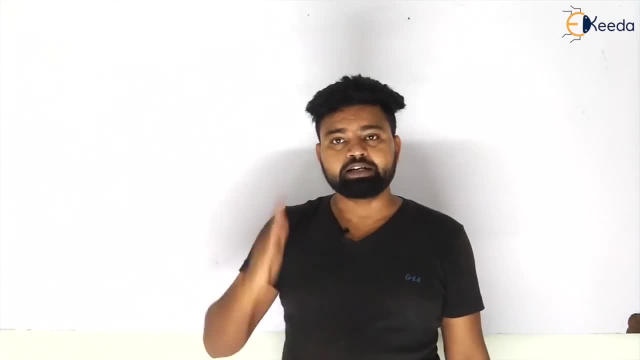 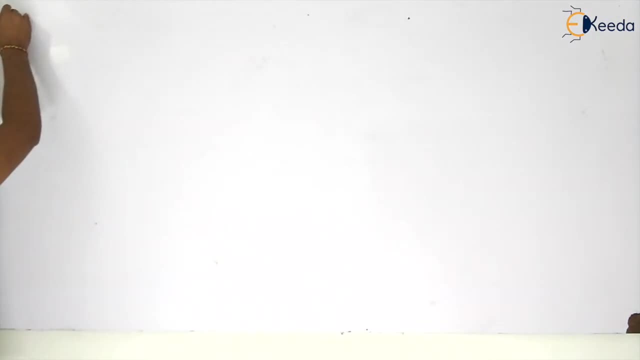 you can calculate the net radiation heat action between the two black surfaces. serial values will be given so. So now we will be discussing about the net radiation heat exchange between two gray surfaces, that is, your non-black bodies. Let us see and focus on the board. my dear friends. 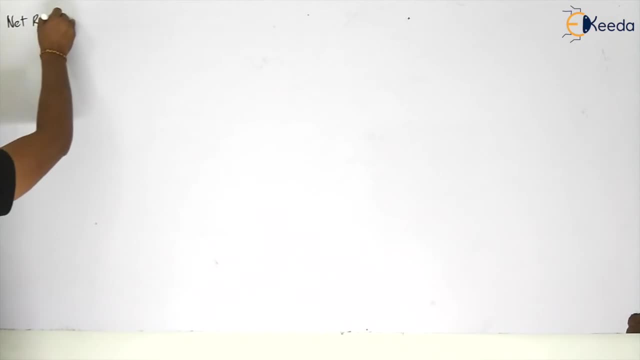 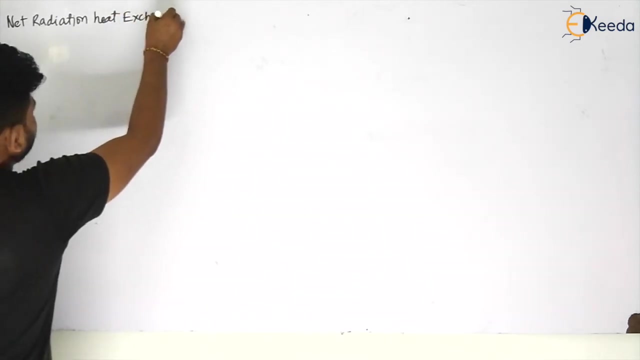 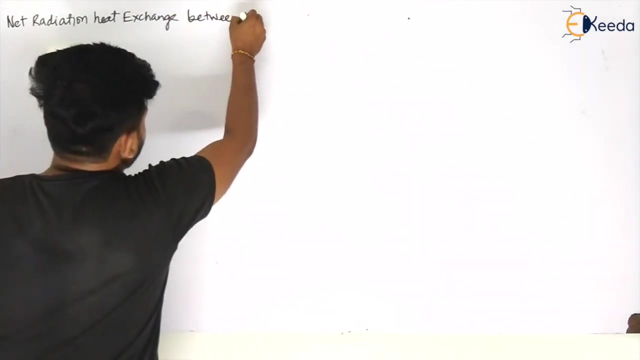 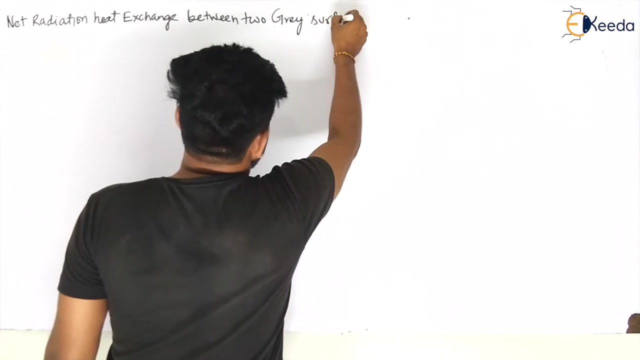 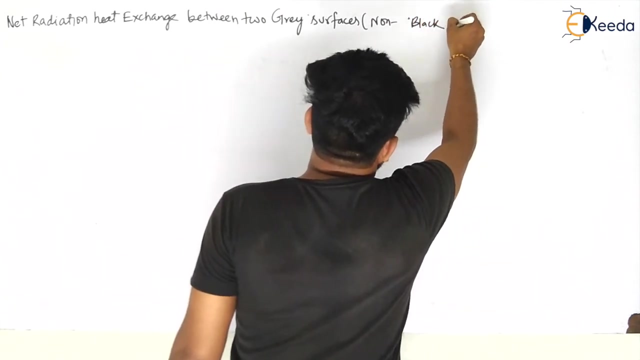 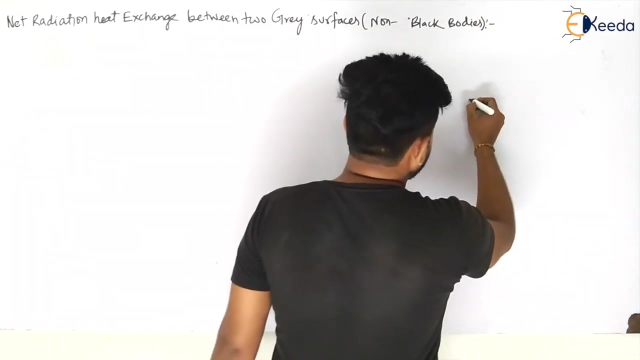 So net radiation heat exchange. it must be radiation exchange, but I am taking radiation heat exchange to simplify this: Heat exchange between two gray surfaces, my dear students. gray surfaces or we can say non-black bodies, non-black bodies. So let us consider two surfaces, let us consider that is your surface one. 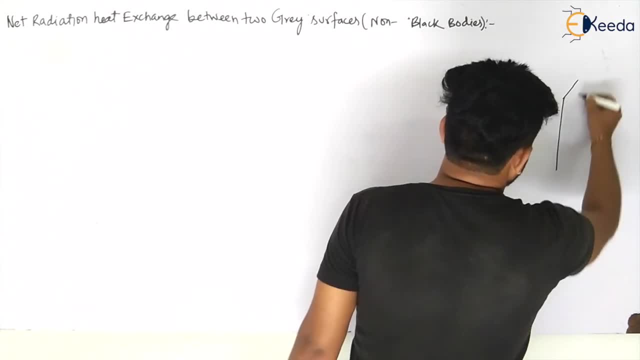 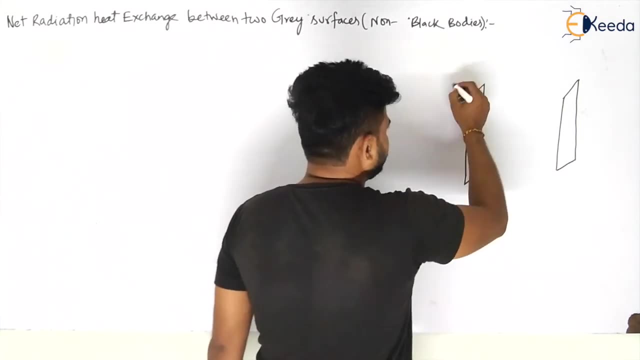 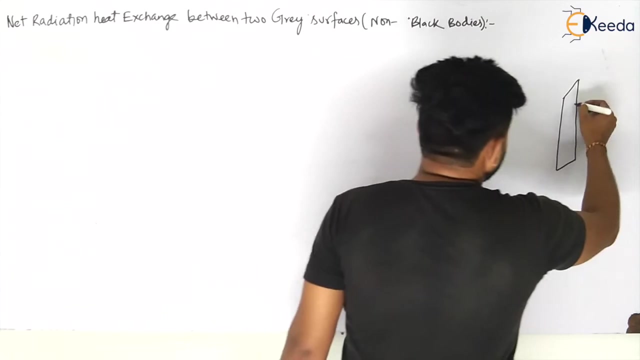 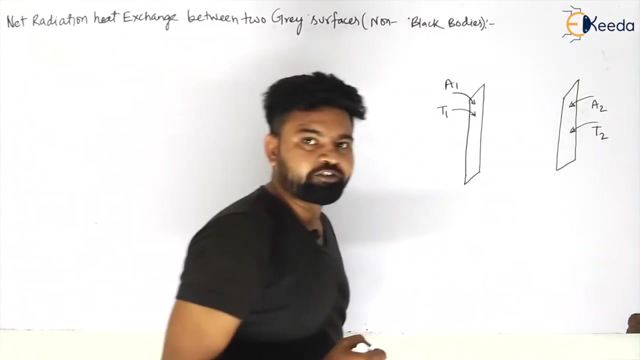 And that is your surface two, my dear students. that is your surface two. Let us take: the area of this particular surface is A1 and temperature of this surface is T1, my dear students. Similarly, area of this is A2 and this temperature is T2 for this surface. 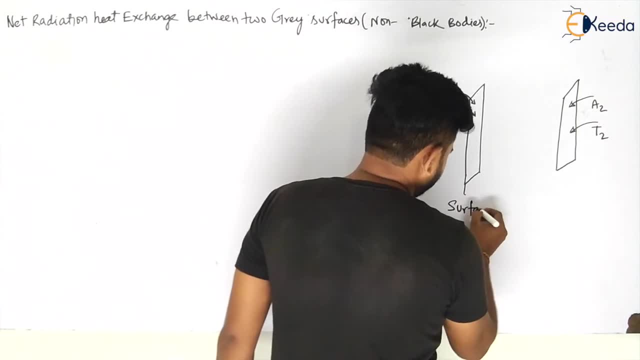 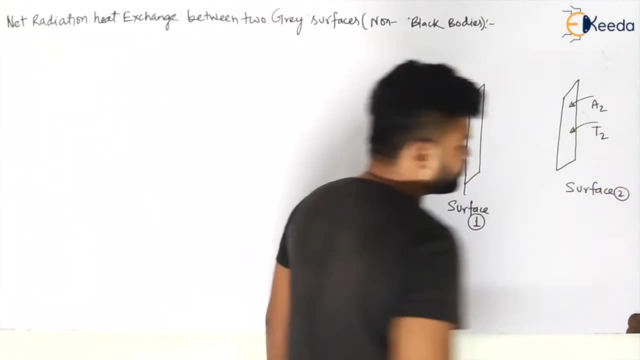 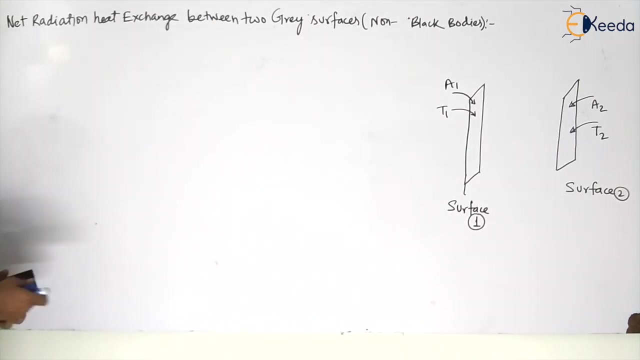 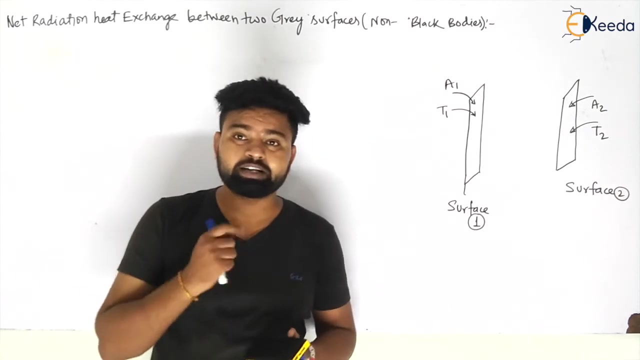 Now, and I am considering, that is your surface one, That is your surface two, surface two, my dear students, okay, Now let us see. let us see. So can I calculate? okay, I know. So how can I calculate the total emissive power of that black body, or that is non-gray? 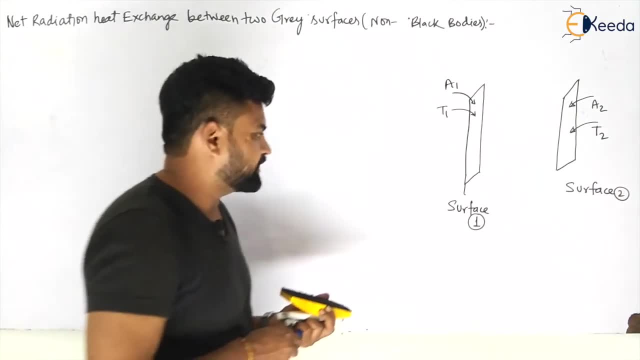 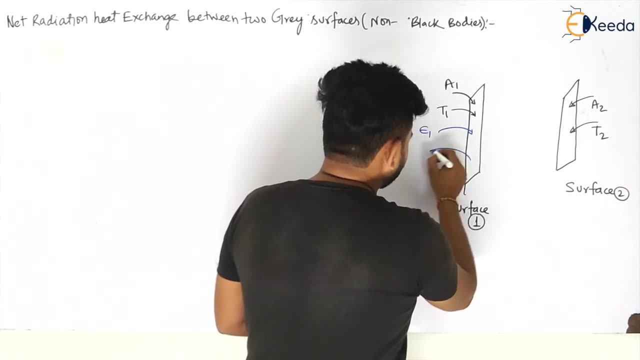 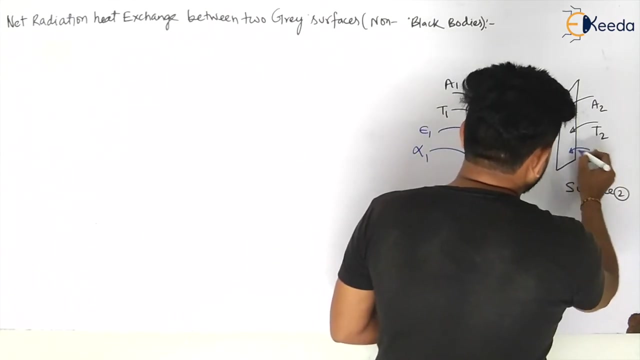 body. So now you have to consider two things also, and these are that emissivity of this surface is T1, my dear students, And absorptivity of this surface is alpha one. Similarly, as these are the non-gray surfaces, emissivity of this surface is E2 and absorptivity 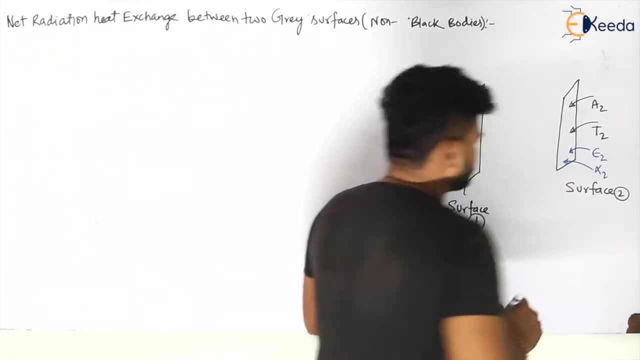 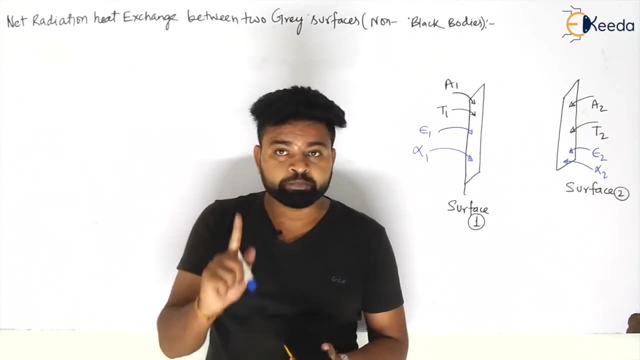 of this surface is alpha two. my dear students, Now, these are not black surfaces, because for black surfaces, E is equal to alpha is equal to one. We know that. But in this case, when we are considering the non-gray surfaces, when we are considering 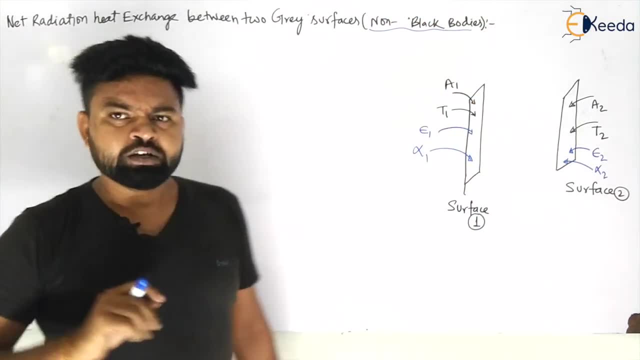 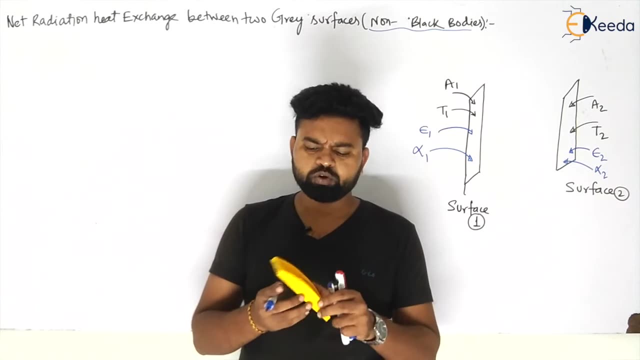 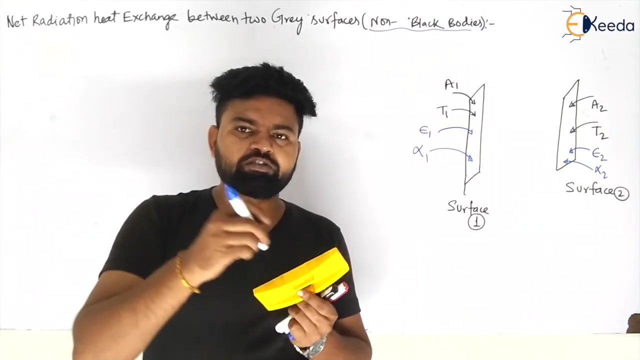 the non-black bodies, Then there will be some emissivity. Okay, So let us feel the concept. what will happen? Let us say: this is your some gray surface. Let us take that is your gray surface. So from this surface, my dear students, there will be emission of radiation. 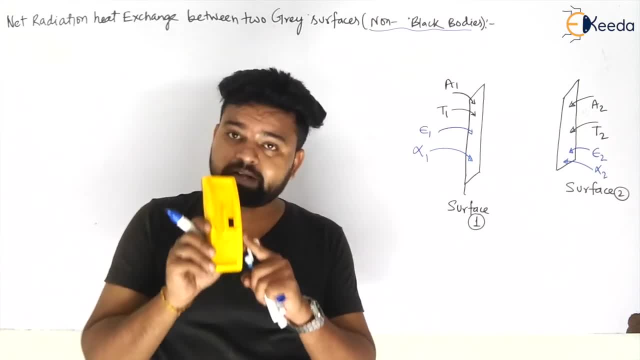 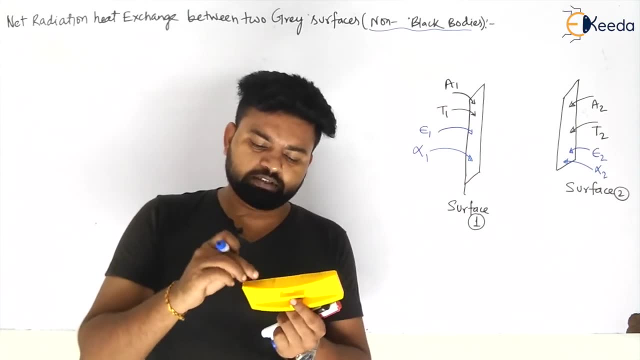 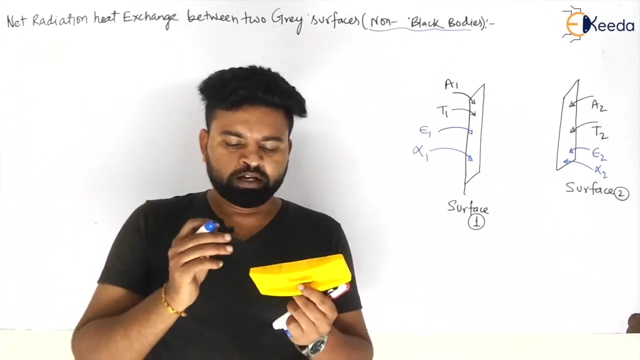 So number of waves are emitting from this? actually, this is having some temperature T above zero kelvin. Let us take it like 300 or 320 kelvin something, So it will radiate in all directions. Yes, So this is non-gray surfaces. that is smooth like okay. 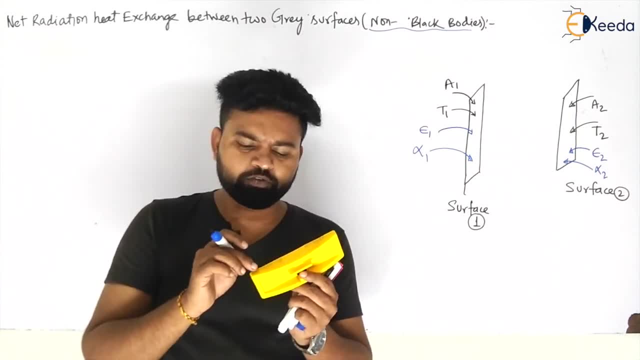 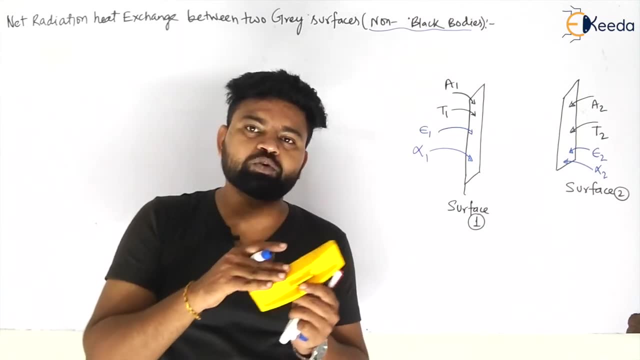 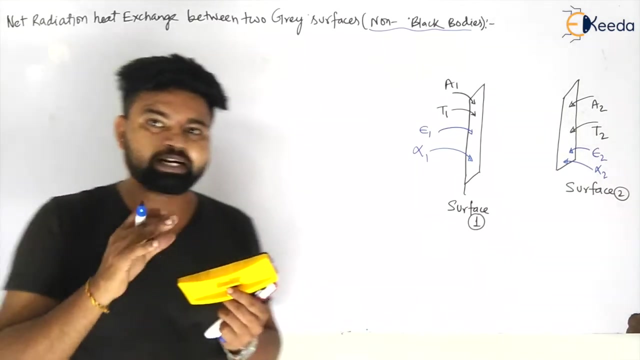 Now, when this will emit some radiation, when this will emit some radiation, what I will do first is I will convert it, or I will imagine that that body is what a black body. So I will calculate the emissive power of this body to be like a black body. 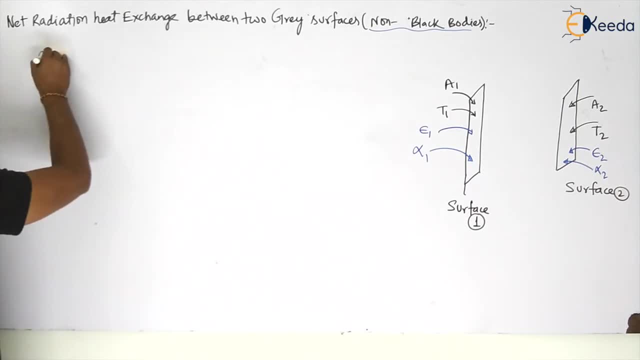 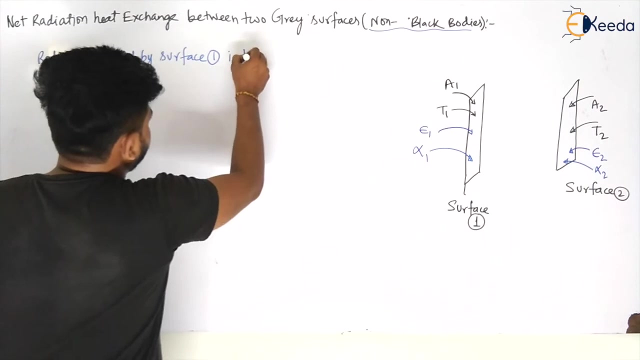 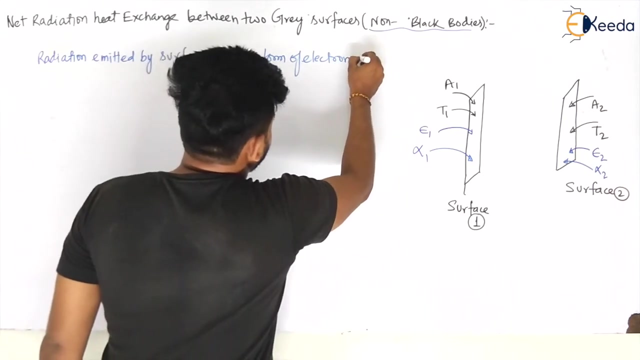 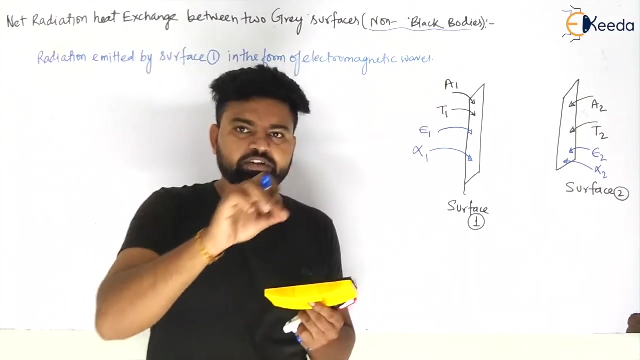 So radiation? So this will be emitted by a surface, one surface one in the form of electromagnetic waves. electromagnetic waves, my dear students. electromagnetic waves, because there will be some emission of electromagnetic radiation. radiation waves, electromagnetic waves. Okay, So I will put this in the form of electromagnetic waves in all directions. 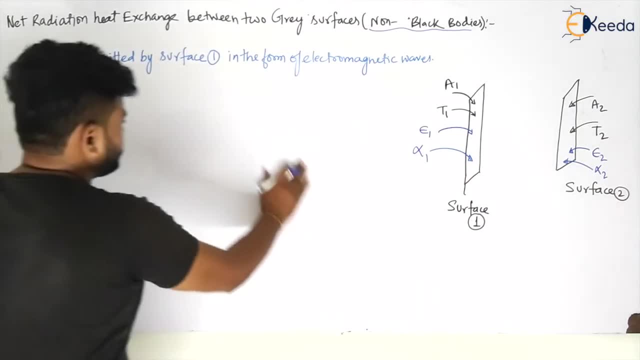 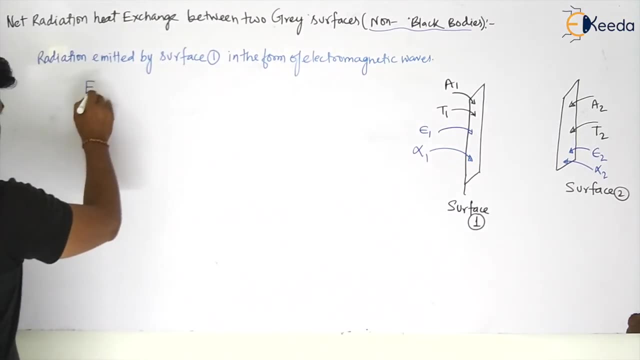 Okay now. So first of all, I will consider it to be like a black body. So what will be the radiation heat exchange? so net radiation, net radiation heat. sorry, I am not talking about that exchange. So the net radiation emitted via this will be or radiation emitted by this body. let us 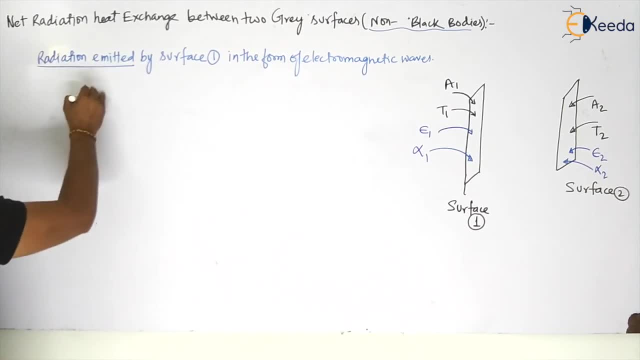 take it. let us say now: let us take layer E1.. E1 is equal to, if it is a black body, E1b is equal to E2.. T1B is equal to. it will become sigma A1, T1 to the power 4.. 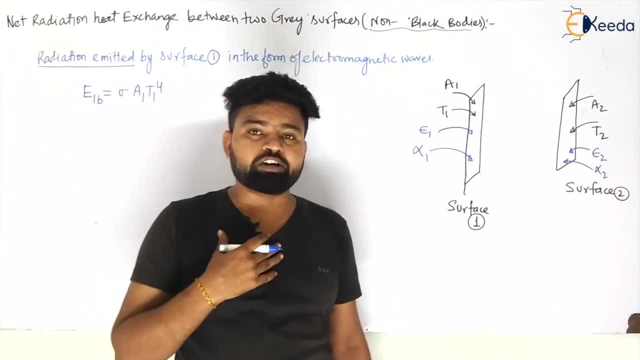 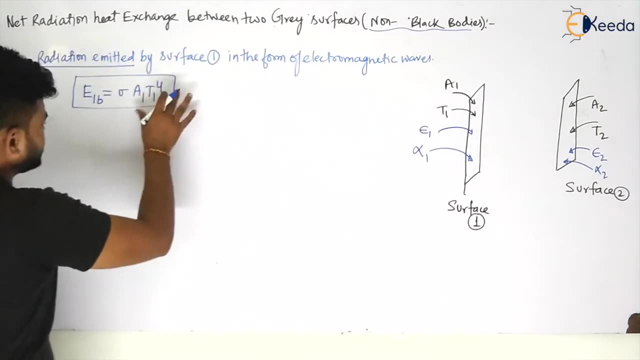 T1 to the power 4.. So, but I want to calculate for the non-blackbody, my dear students, non-blackbody, So that is for blackbody. This net radiation, that total emission by the blackbody is this: 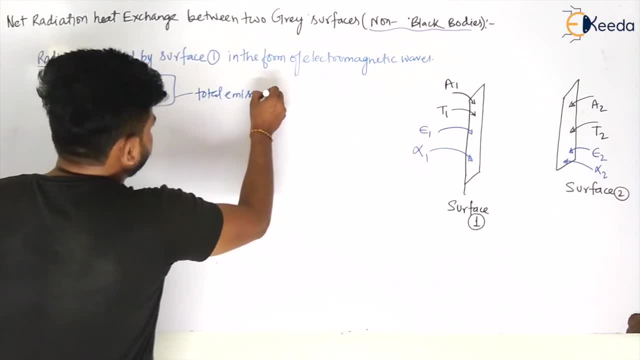 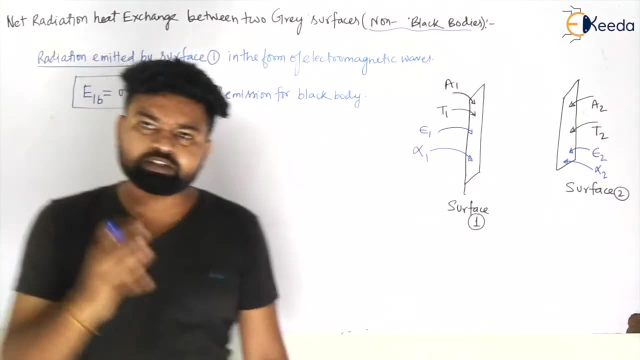 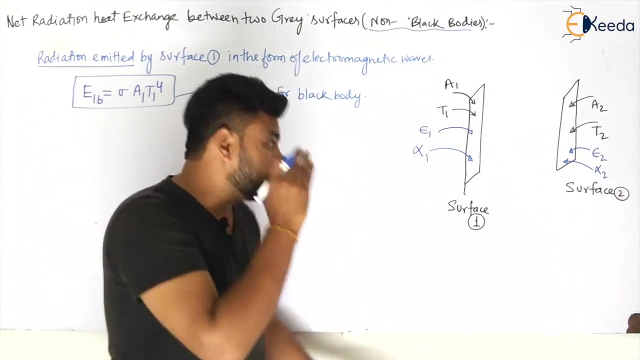 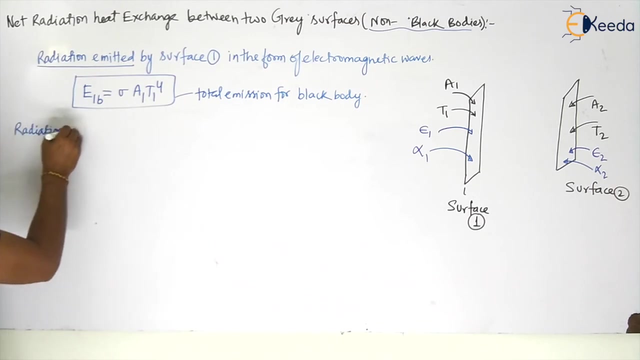 That is total emission for blackbody, For blackbody. So by comparing with the blackbody, now I will, I will calculate the net, I will calculate the radiation, heat exchange, or radiation emitted by surface. one, my dear students. So radiation emitted by gray surface. radiation emitted by gray surface. 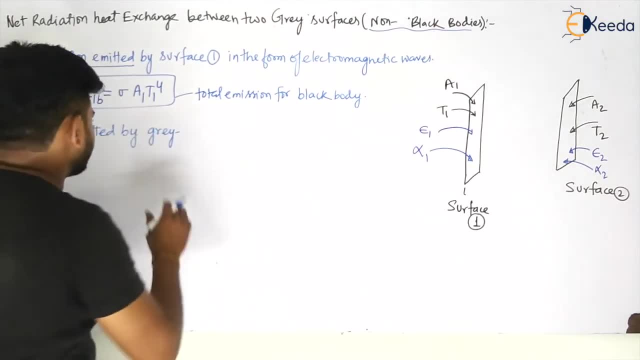 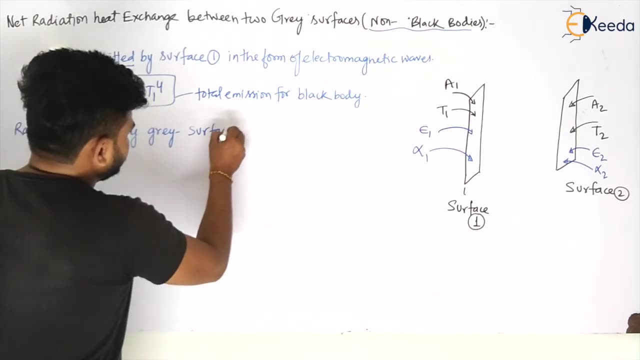 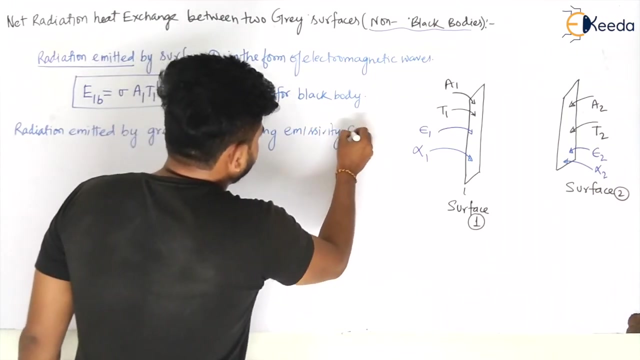 This is very important concept. that is why I am going slow. my dear students, So carefully, just learn it. So radiation emitted by gray surface. So having emissivity, having some emissivity, let us say E1, okay. 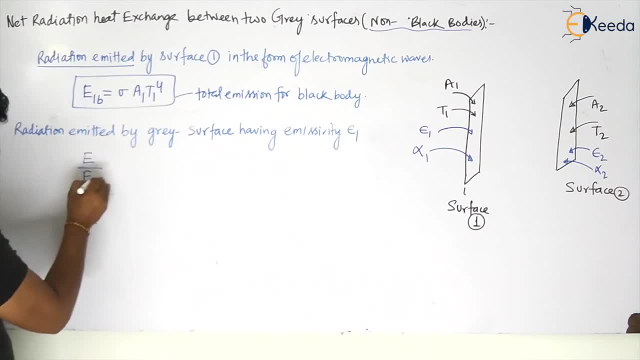 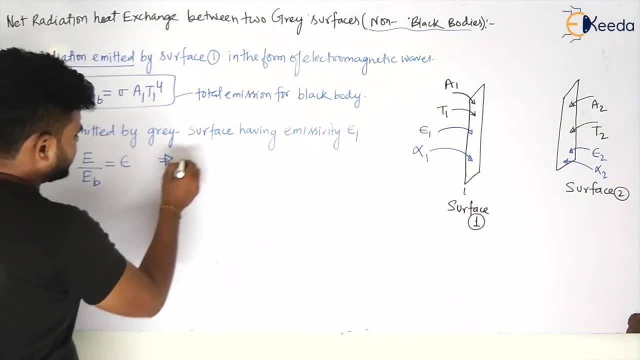 So we know already that E by EB is equal to emissivity. E, my dear students, yes or no, We know that. So for a gray body, I can easily calculate E1.. Yes, I can calculate E1.. 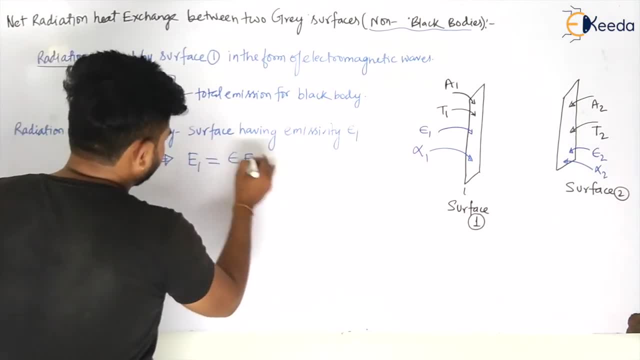 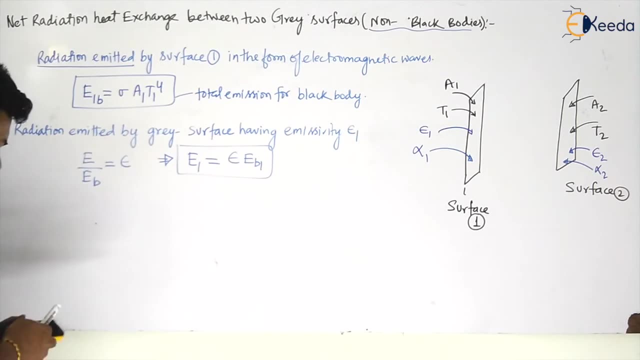 So this will become E of EB1.. Yes or no? Now, what will be the? The radiation emitted by this body, my dear students? that is, that is surface 1.. So this will become equal to. E1 is equal to E of, that is E1, sigma E1, E1 to the power 4,, my dear students, E1 to the power 4.. 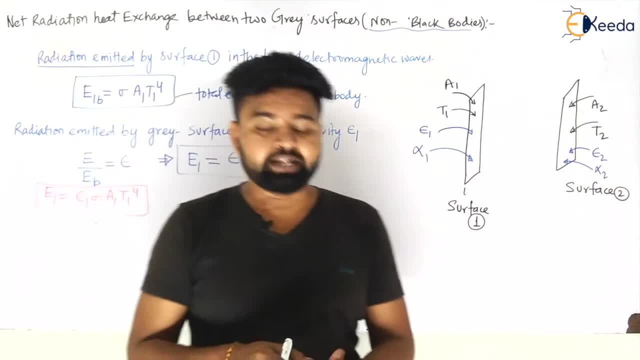 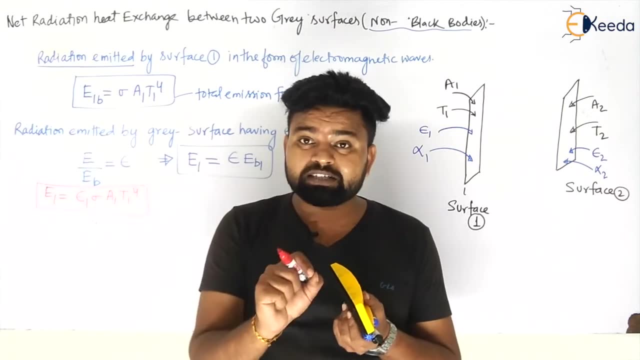 So this will be the radiation emitted by the body, because that surface will decide that how much radiation I have to take, because it is having some kind of what Emissivity. So let us say, if it is emitting 100%, 100 rays, it is emitting. 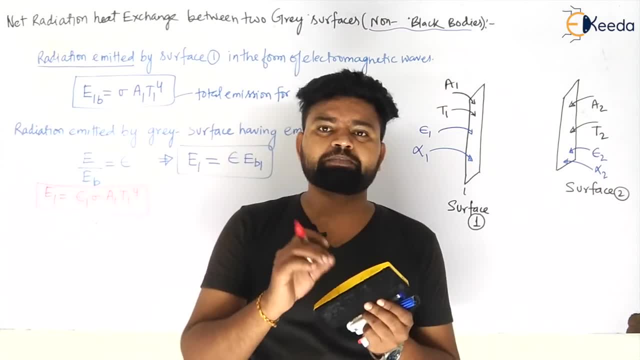 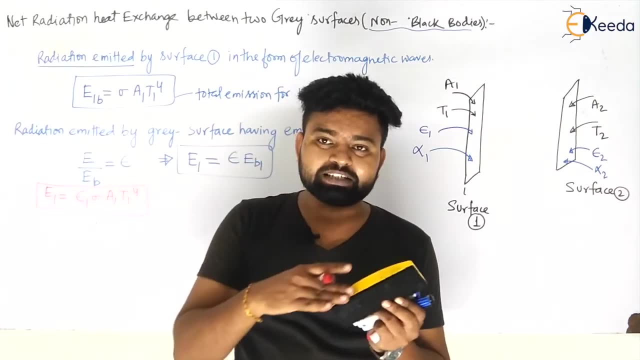 But that is having some emissivity. let us say 0.9, 0.9.. So what will happen? Only there will be emission of 90% rays from this surface. Hope you are getting that feeling now. So there will be what emission of? 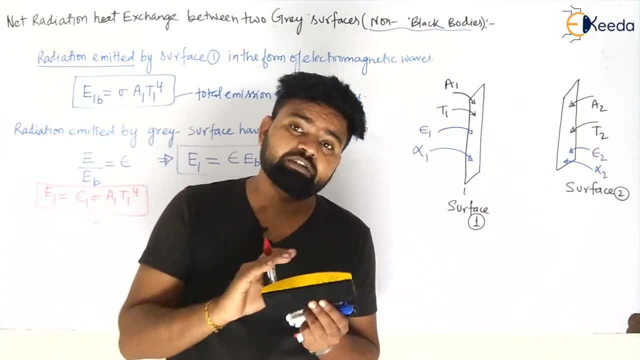 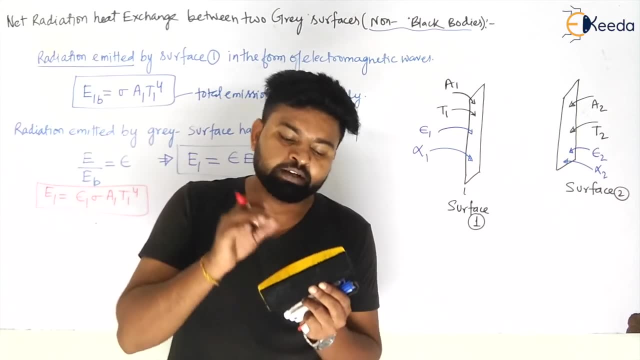 90% waves. So I have to take compared to the black body. if it is a black body it is emitting 100%. then if the other surface, not the surface, is having some emissivity, then this surface, compared to this black body, is emitting what? 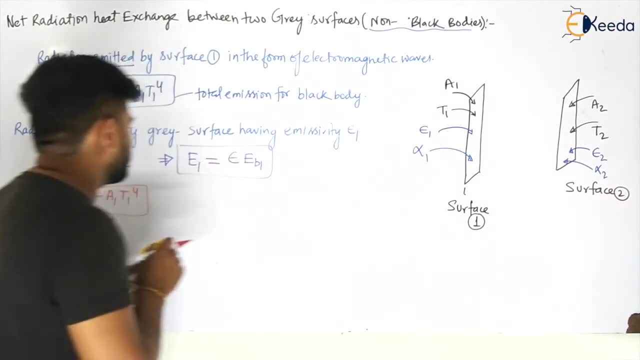 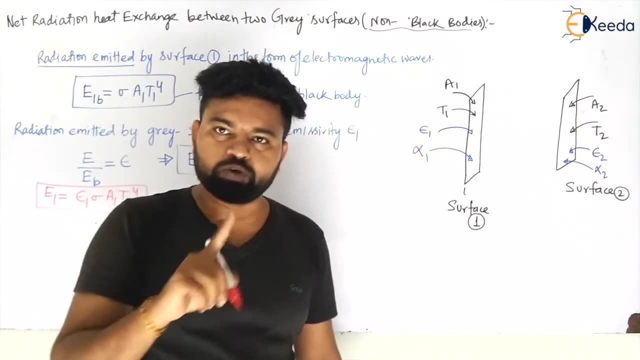 100%, But 90%, 90% or 90% or with some emissivity, my dear students, because for black body emissivity is 1. So all the gray surfaces will be having the emissivity less than gray, less than your black body. 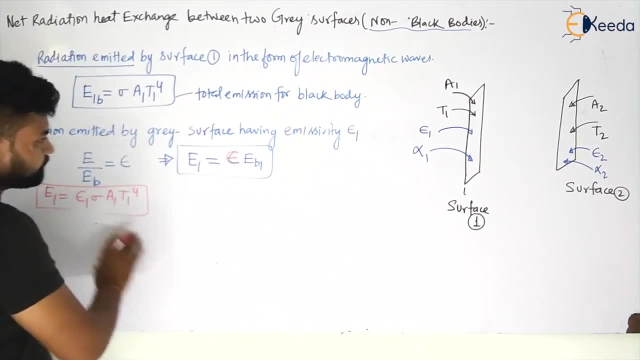 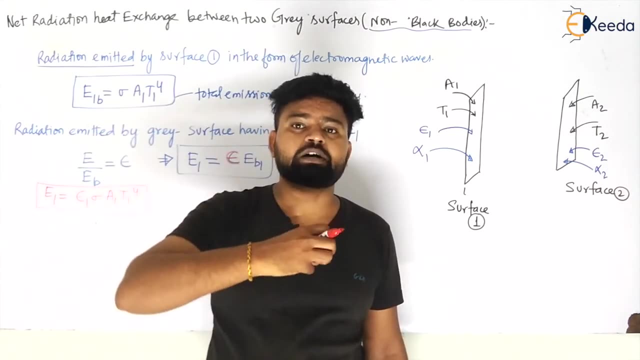 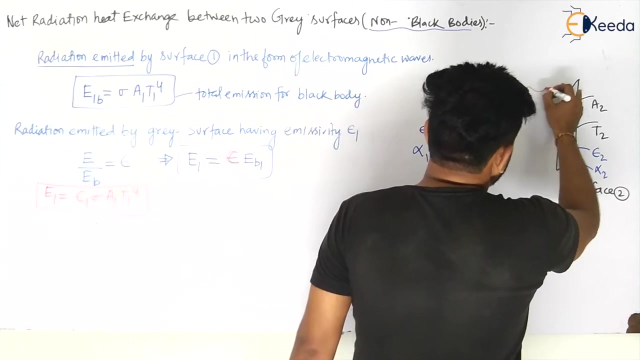 So now we know that how much it is radiating. Okay, Now I want to know that the radiation which is transferred or which is coming out from surface 1. Is going Or absorbed by surface 2.. So some radiation is going out from this. 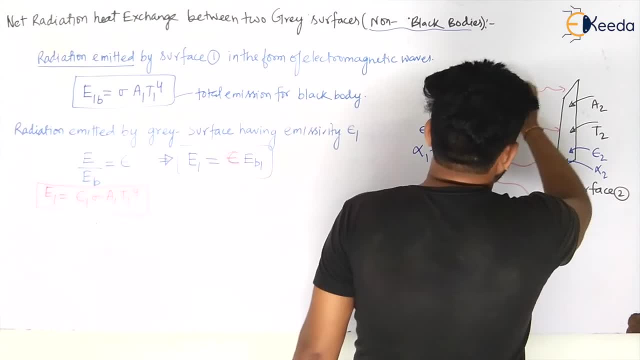 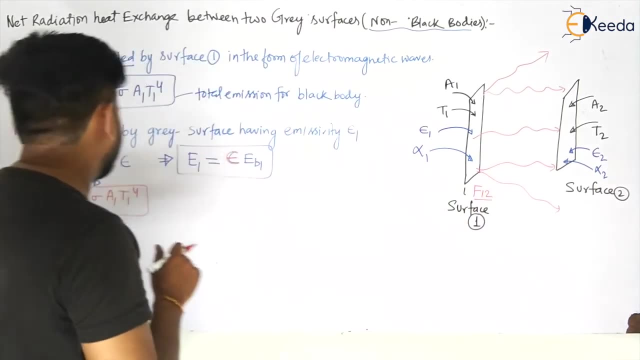 And absorbed by 2.. Some is going out. Some is going out, my dear students. So what will be this? This will be F1, 2. It will tell. a shape factor will decide. Okay, Now the radiation. 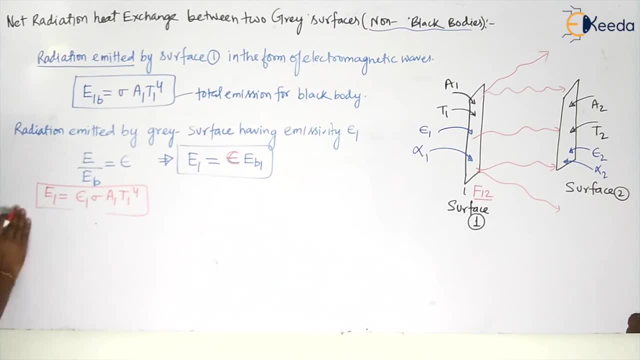 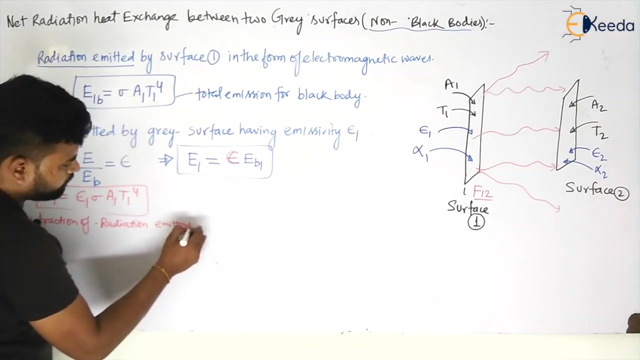 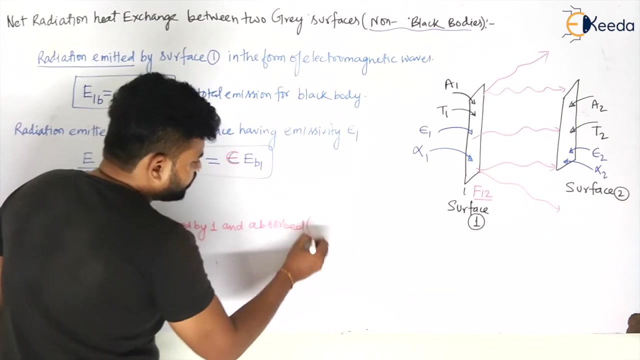 The radiation, Or we can say the fraction of radiation emitted by 1 and falling on 2.. The fraction of radiation emitted by 1, by 1 and absorbed by 2, absorbed by 2. And which factor will decide that it is absorbing? 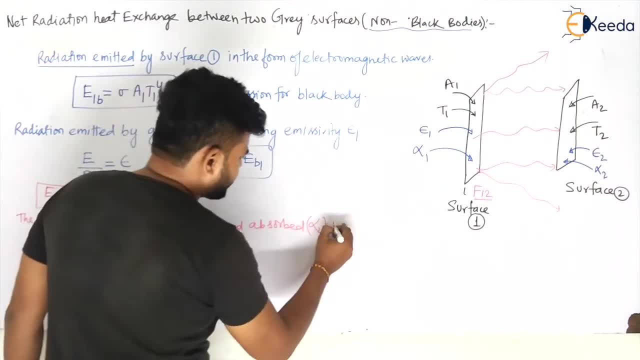 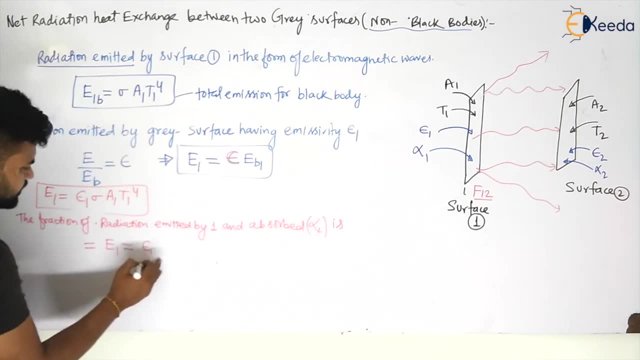 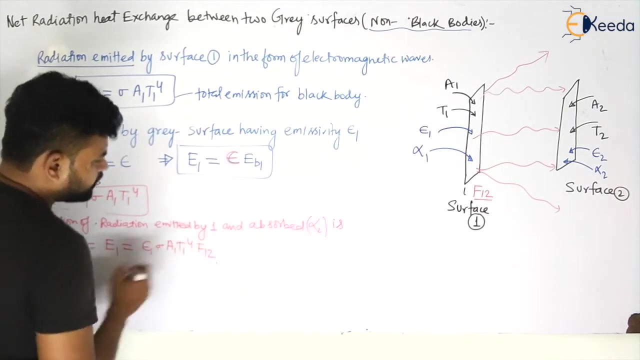 That will decide alpha 2, alpha 2. Absorbed by 2 is equal to, that will be nothing. but E1 is equal to E1 to the power 4 multiplied by F1, 2,. my dear students, 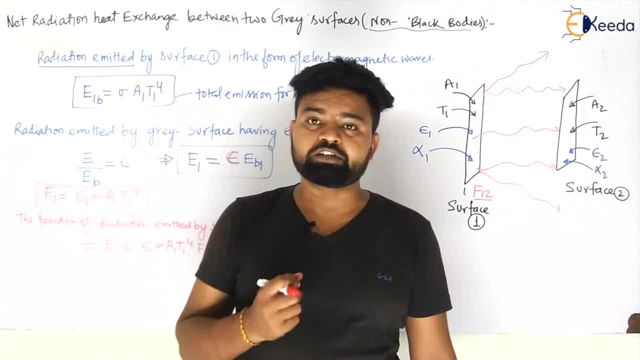 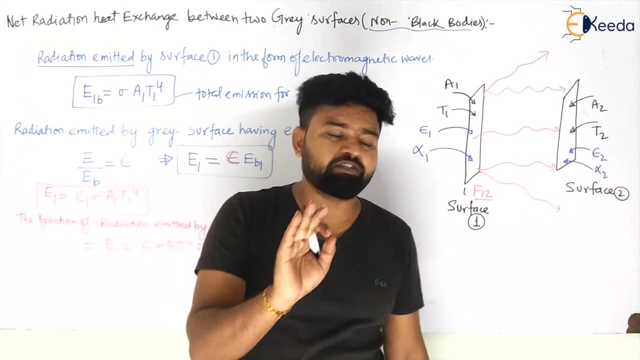 Okay, And now it will only absorb the radiation which is falling on that, And that factor, that is absorptivity, will decide that how much it is absorbing, If this is having, let us say, absorptivity 0.5.. 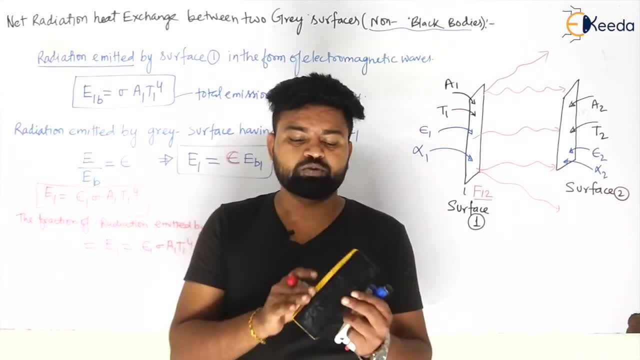 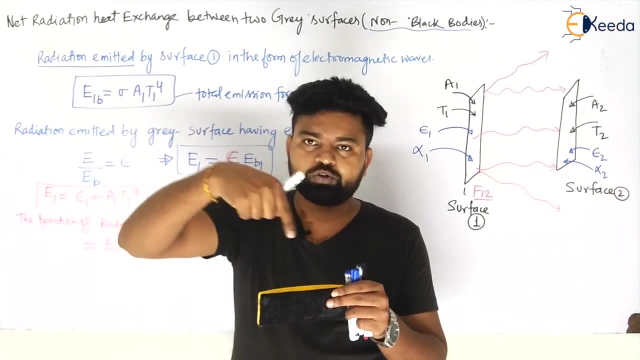 Then it will absorb only 50% radiation like this. So if, like other surfaces there, And if it is absorbing, The sum of radiation is falling on that like this- Okay, Falling on that- like this, Electromagnetic waves are coming and falling on this. 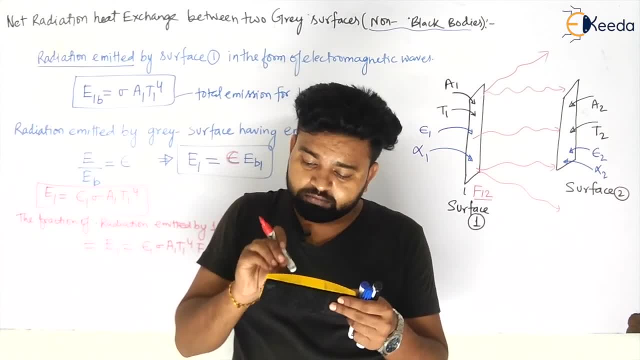 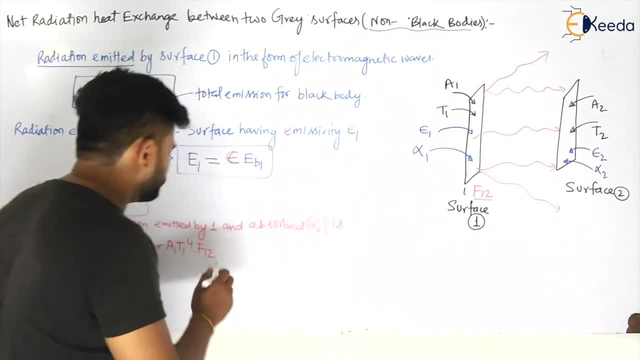 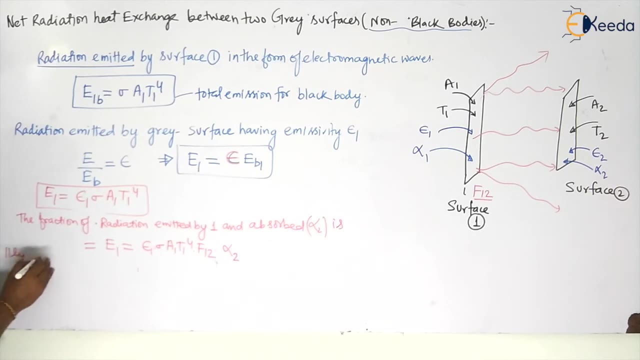 So it will only absorb the radiation Which will decide that absorptivity, will decide that how much radiation it will absorb. So that is why you have to say alpha 2 also, my dear students. Similarly, similarly, similarly for, similarly for body 2 or surface 2 we can take. 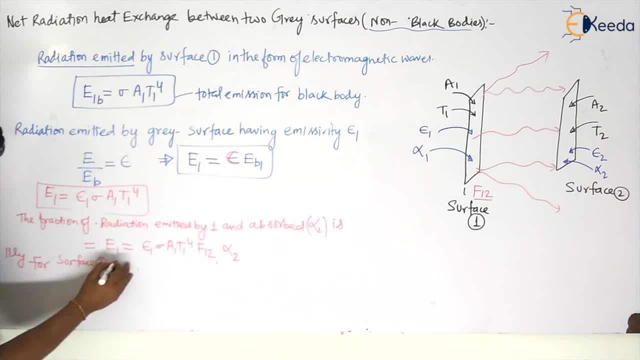 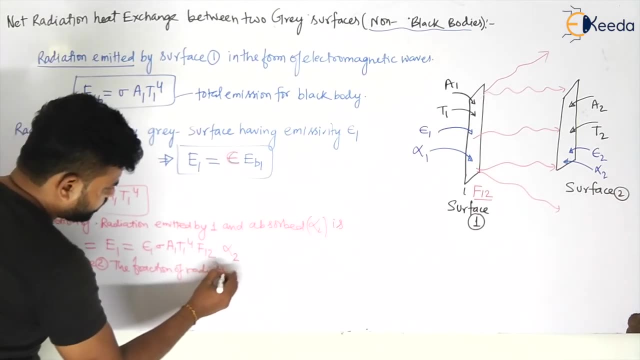 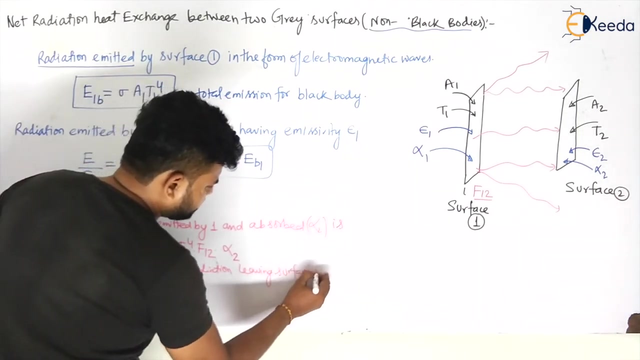 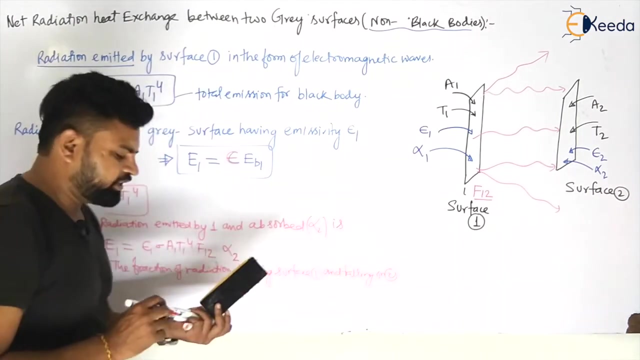 Surface 2, surface 2, the fraction of radiation, the fraction of radiation coming out or leaving surface 1, leaving surface 1 and falling on 2, falling on 2,, my dear students. So the fraction of radiation which is leaving surface 1 and falling on 2, can we calculate this? 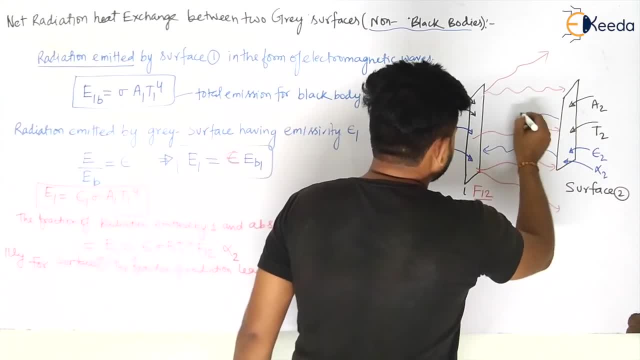 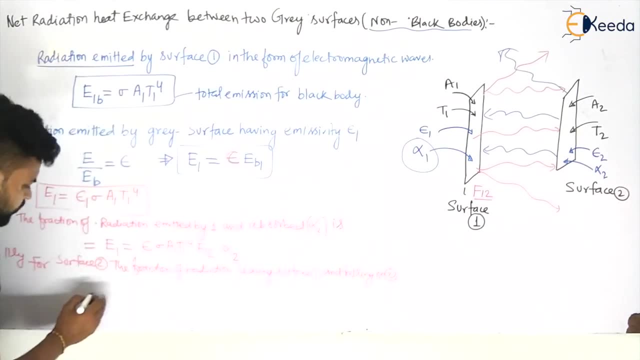 Yes, sir, We can calculate How. So this is coming out from the surface 1 and falling on 2.. So this is also having some absorptivity. alpha 1,, my dear students, Yes or no. So can I calculate the E2 directly now? 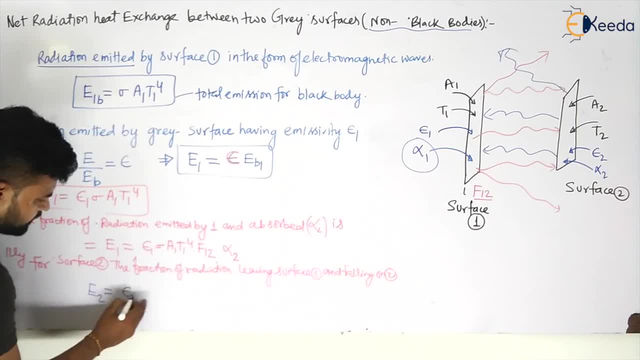 So the E2 will become equal to That is that will the initiative will decide that how much it is coming out from this second surface with the black body, That is nothing but sigma A2. E to the power 4 multiplied by F12.. 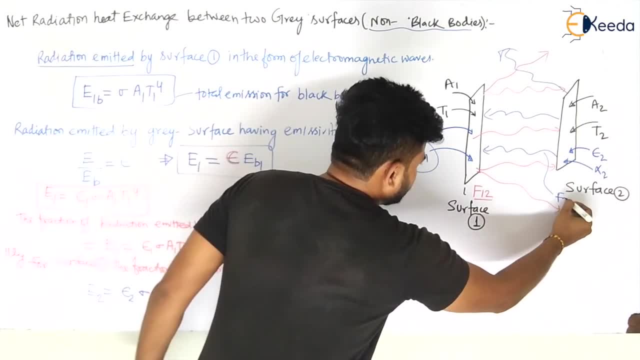 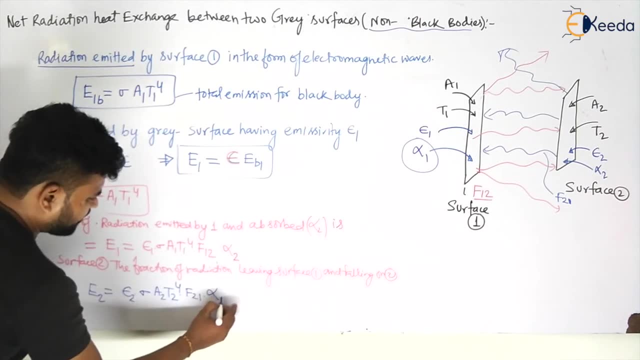 That is what, my dear students. the fraction of radiation will be leaving 2 and falling on 1.. That will be F21 multiplied by alpha 1 will decide. alpha 1 will decide, my dear students. So now I know E1 and E2.. 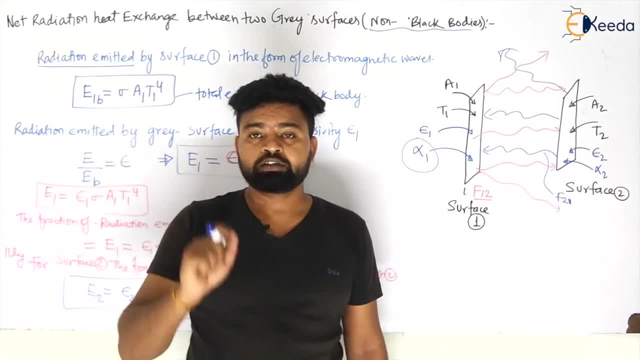 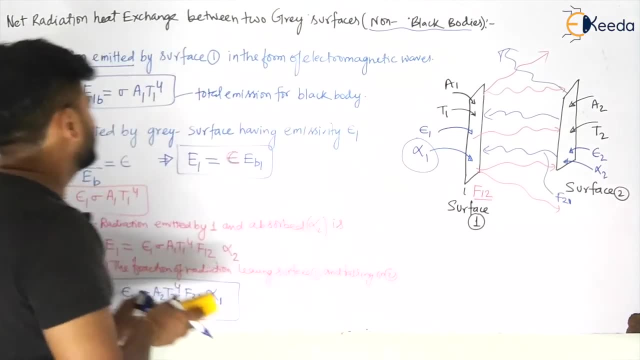 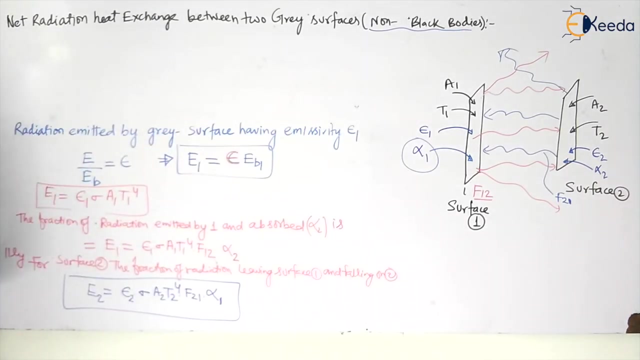 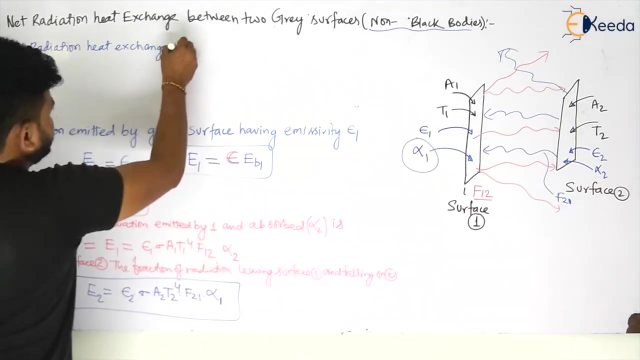 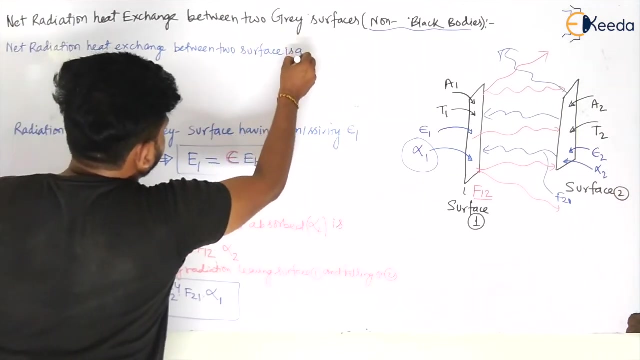 So can I calculate the net radiation heat exchange, or net radiation or net heat exchange between the two non-gray surfaces? that has calculated. So the net radiation Exchange between two gray surfaces will be given by. So the net radiation heat exchange between two surfaces is given by. 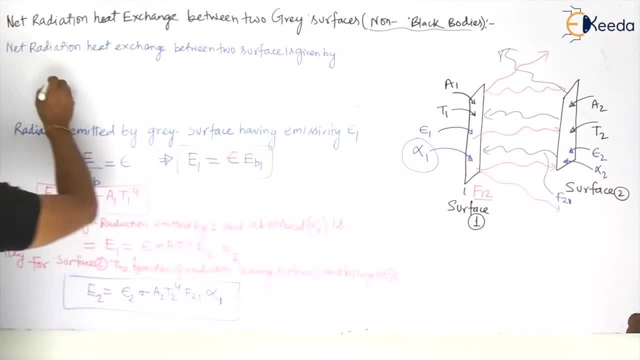 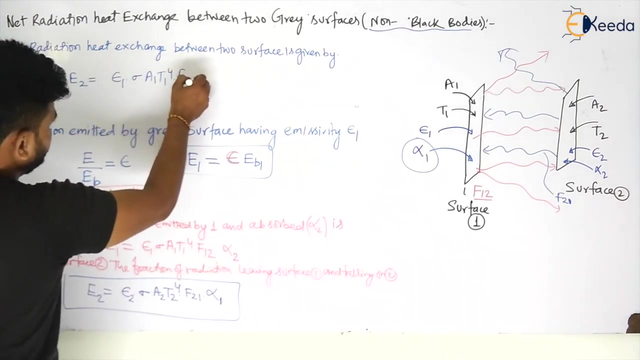 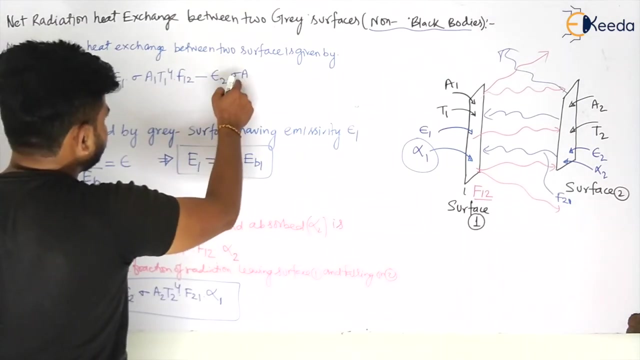 That is your E1.. E1 minus E2,, my dear students. So this will be what E1 is. how much. That is epsilon 1.. That is E1 sigma A1, T1 to the power 4 into F12, minus E2 sigma A, sigma A to T to the power 4 into F21,, my dear students. 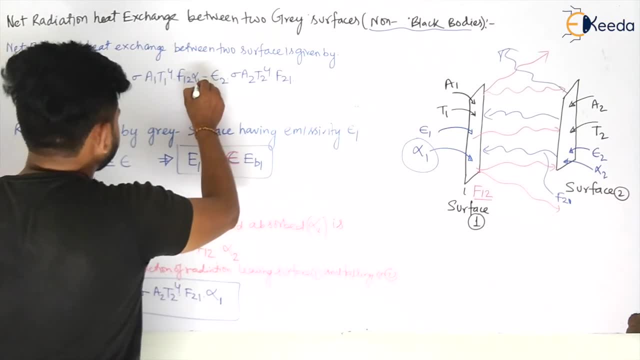 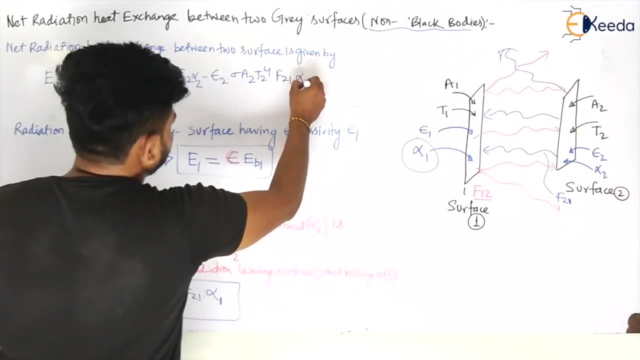 And I have not taken alpha 1.. Let us take alpha 1 here. In this case, this will be alpha 2.. Alpha 2. In this case, this will be alpha 1.. This will be alpha 1.. So now, using the reciprocatory theorem, what you will have? 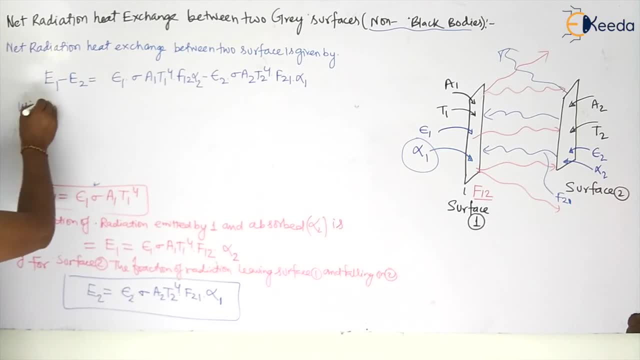 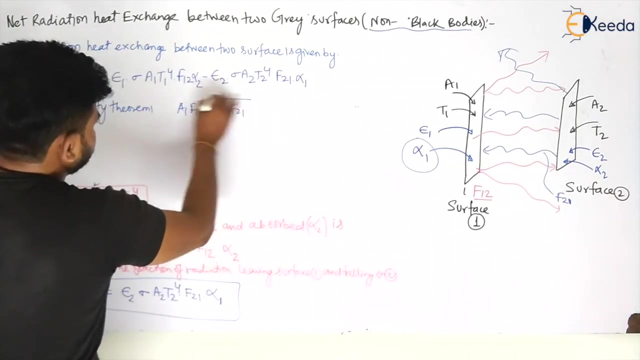 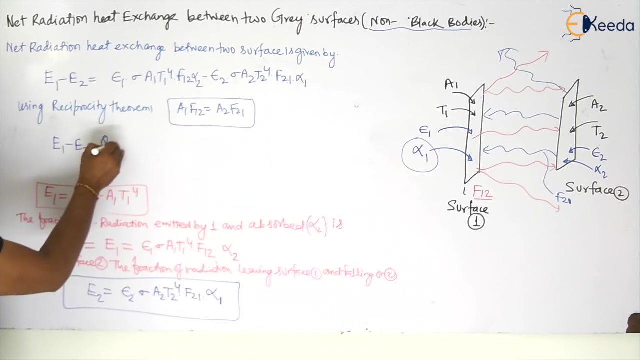 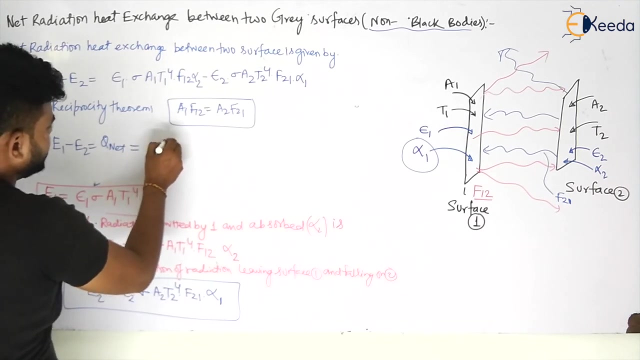 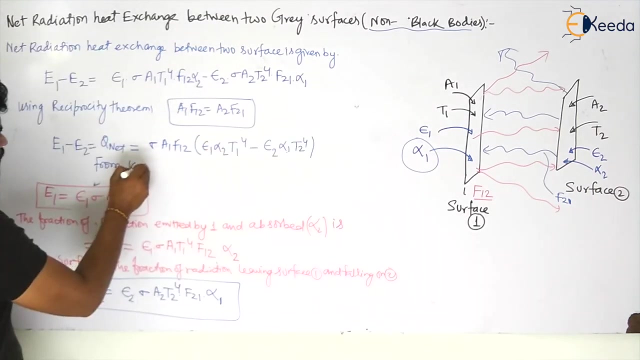 Using the reciprocatory theorem. So using reciprocatory reciprocity theorem it will be. We know that A1- F12 will be equal to A2.. F21.. Now, replacing this with this value, I will have E1 minus E2, or that is Q. net will be given by sigma A1- F12 into E1 alpha 2 from Christoff's law under thermal equilibrium. 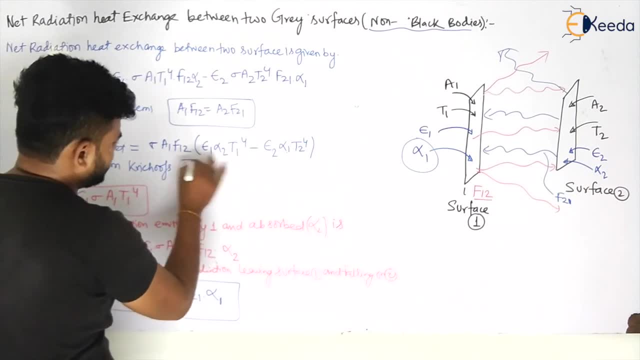 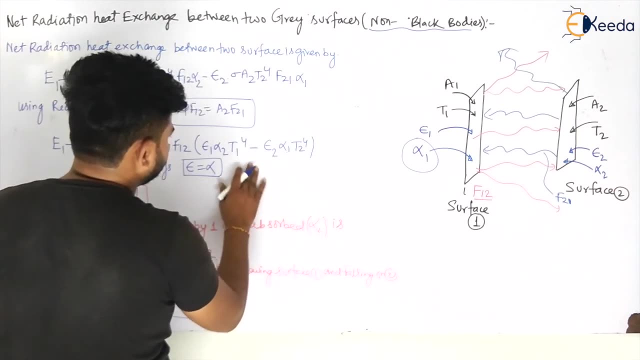 That emissivity is equal to absorptivity, alpha. So can I take that E1? E1, or we can take that, Observe I2.. So this will be: E1 is equal to E is equal to alpha. my dear students, 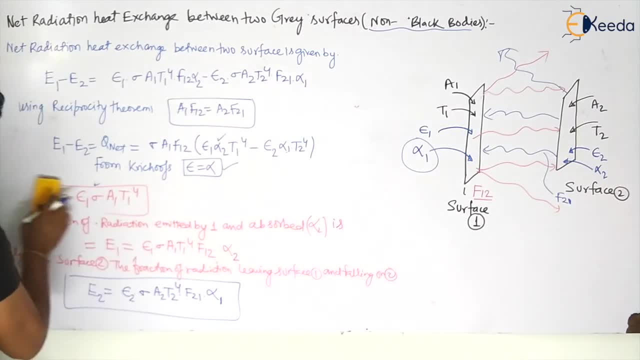 Can I take alpha? Yes, I can take Out, So let us take it. So this will be: That is Q. net is equal to sigma A1, F12 and E will be equal to alpha, So E1.. 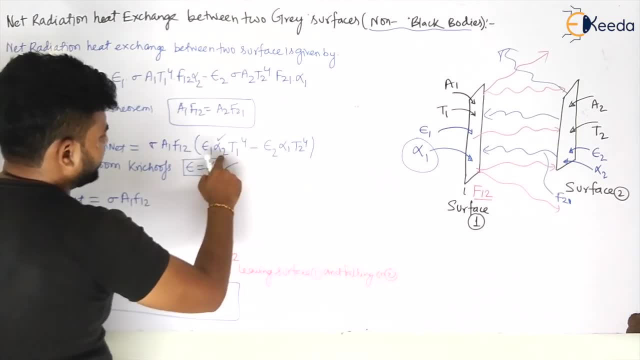 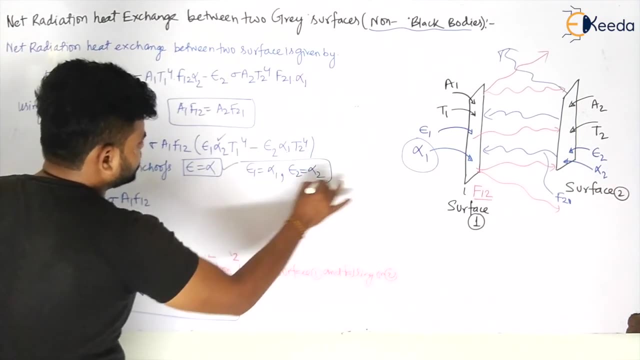 E1 will be equal to What? Alpha 1.. That is E1.. And alpha 2 will be equal to what That is. E1 is equal to alpha 1.. That is E2 is equal to alpha 2.. E2 is equal to alpha 2..